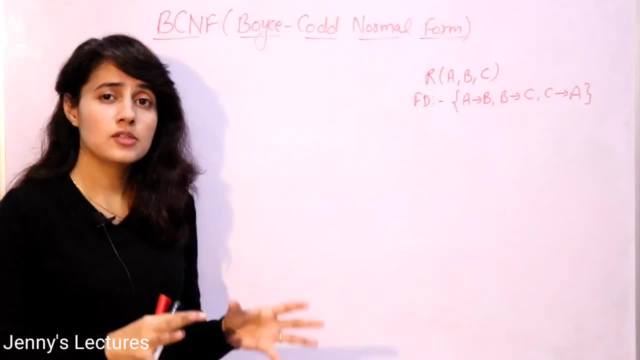 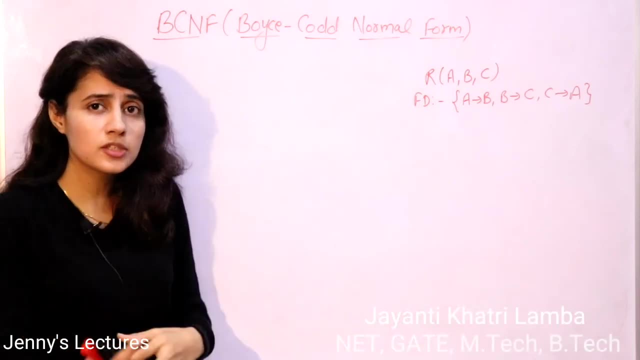 So far in this lecture series of DBMS, we have discussed first, second and third normal form right. What is the basic idea of these? those normal forms means, what are the rules and regulations for a relation to be in first, second and third normal form right, And we have also 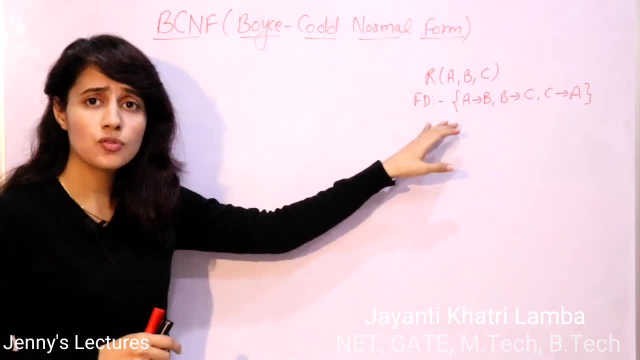 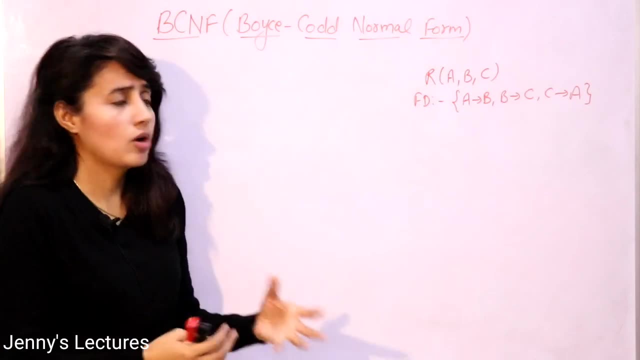 discussed that a particular this type of relation would be given. functional dependencies would be given and you have to identify that the particular given relation is in. you can say in first, second or third normal form or not. right Using those rules. We haven't discussed that. if a relation 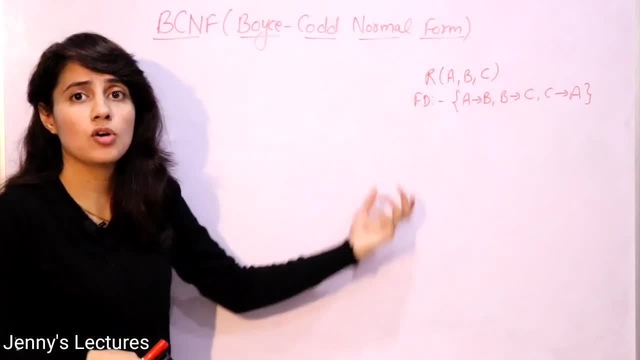 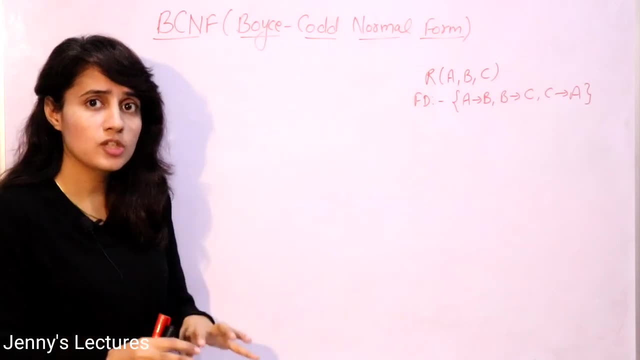 is not in second normal form, then how to convert it into second normal form means how to decompose that relation. Fine, First of all, we will discuss the basic idea of all the normal forms. So in this video I'll discuss what is BCNF. Now, what are the drawbacks in the second normal form? 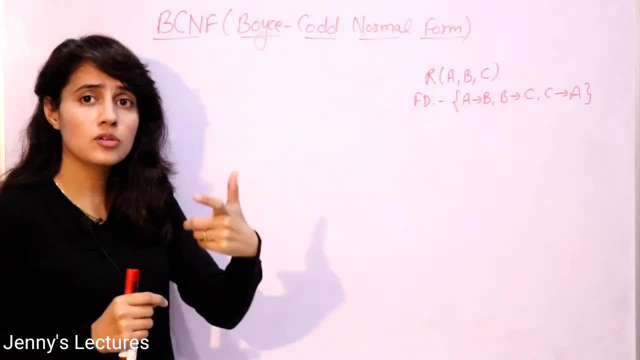 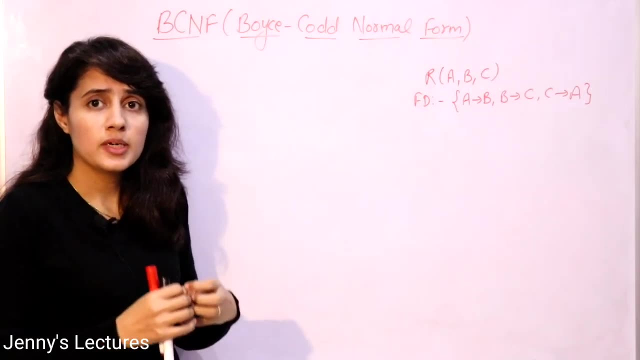 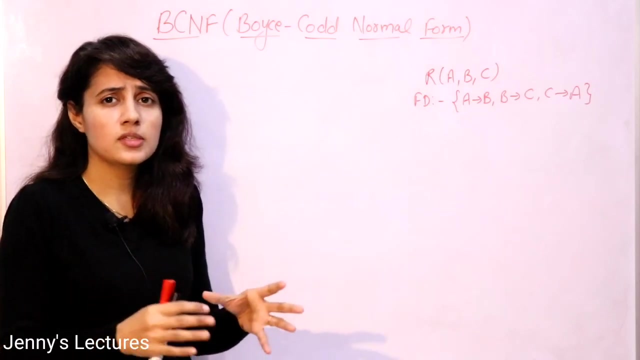 and because of those drawbacks the concept of third normal form came into picture. that also we have discussed in the previous video. right, But still we have some drawbacks in third normal format sometimes. See, I have told you in the previous video that if your database design, your relational schema, is in third NF, then you can say that it is. 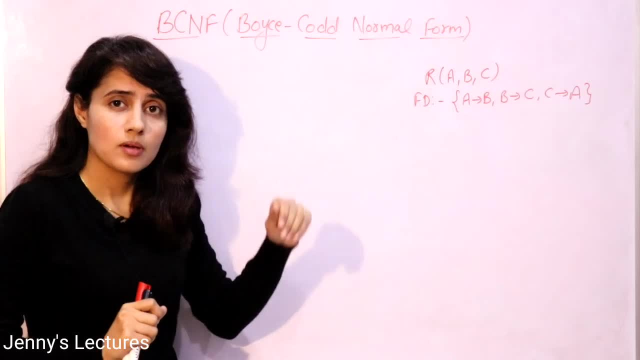 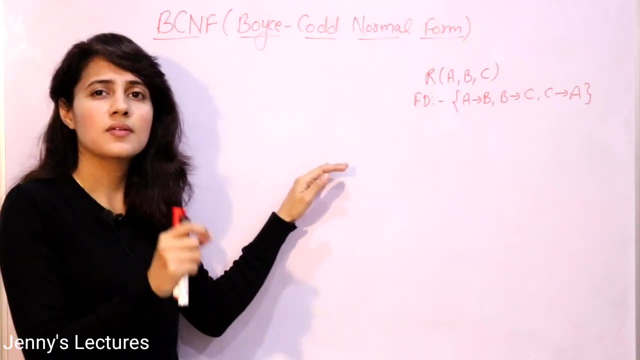 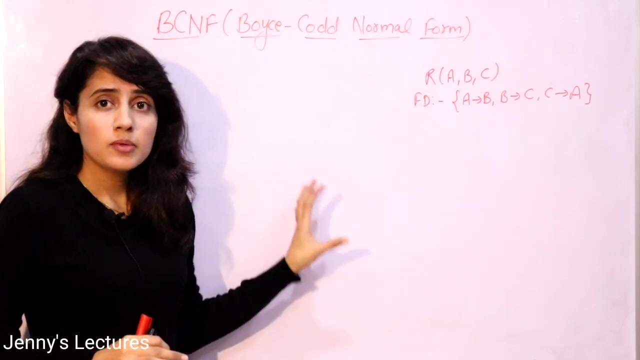 a good database design right, But sometimes still because at some cases still there are some redundancy. if your table is in third normal form but still there is some redundancy exist in that table and because of that you can get some anomalies right When this type of problem 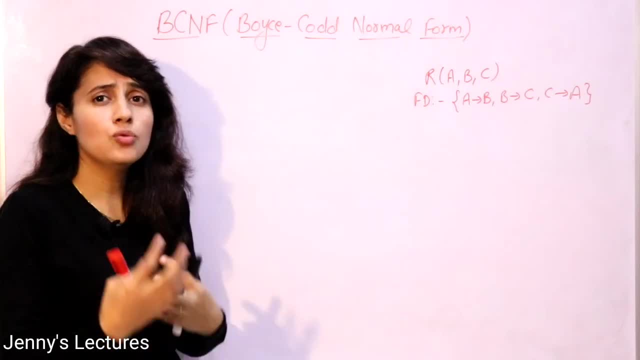 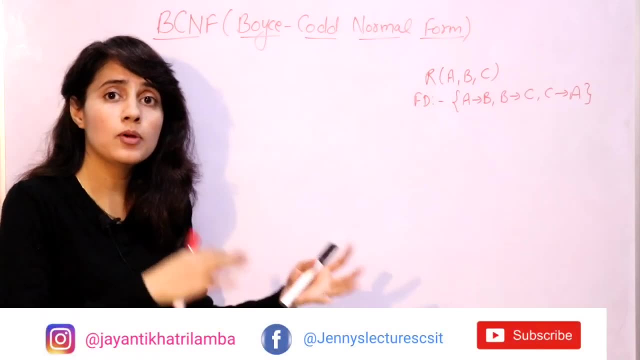 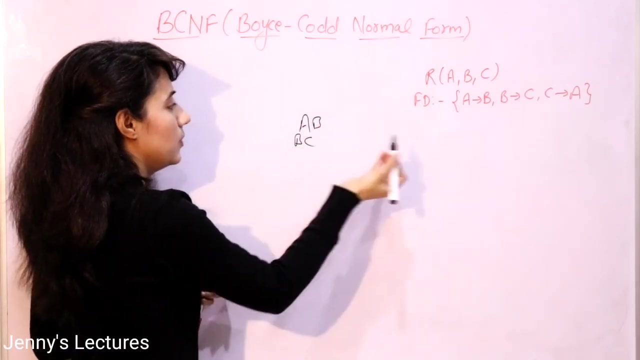 comes because, third, NF you know is not able to handle the cases when you have multiple candidate keys and all the candidate keys are overlapping. or you can say: we have multiple overlapping candidate keys, like this: Suppose, in a relation we have one candidate keys, AB. second is BC. next you can say DC, like this: 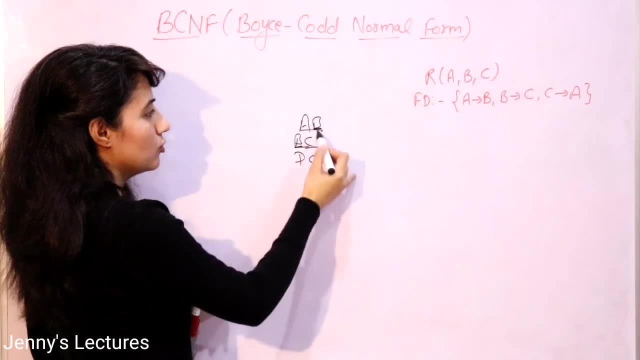 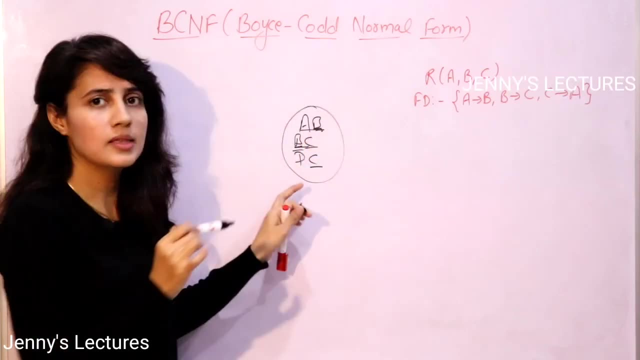 See this and this is overlapping candidate keys: here also C, here also C, here B. here we have B. So when these kind of cases exist, then third normal form cannot handle these type of cases. right To handle these type of cases we have BCNF. 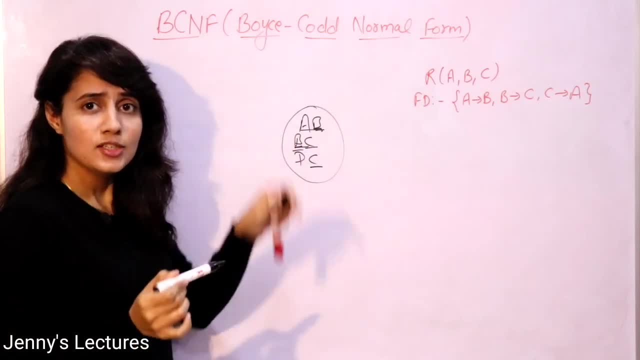 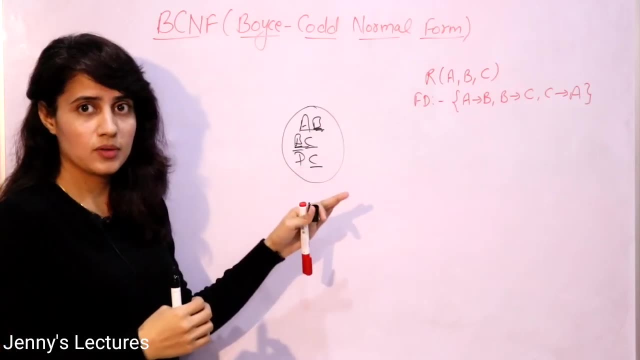 We cannot say that it is 4th normal form. right, It is. you can say that a stronger version of third normal form, or you can say advanced version of 3NF. And why it is known as Boyce-Cord normal form? Because it was developed by EF-Cord. 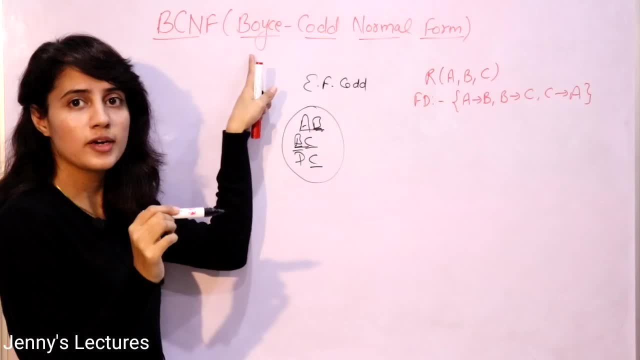 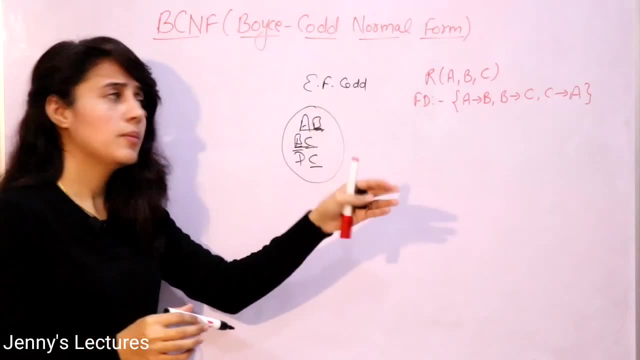 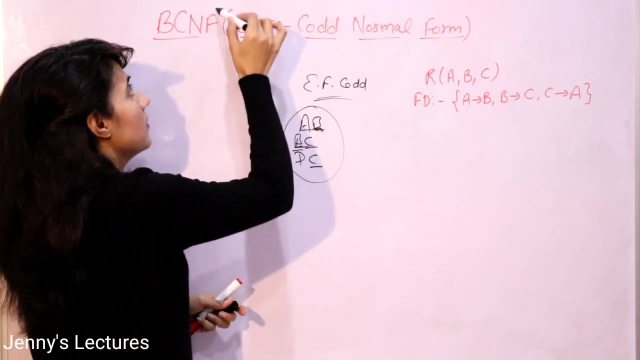 and Raymond F Boyce. That is why it is known as Boyce-Cord normal form. It is not fourth normal form right remaining. first, second and third normal form was developed by ef code. only see he is known as father of dbms right now. why this is more strict than third normal form. 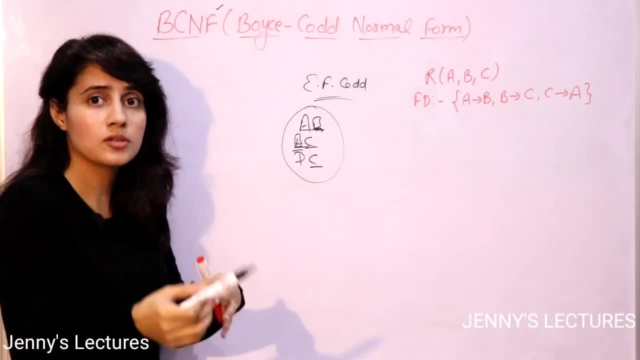 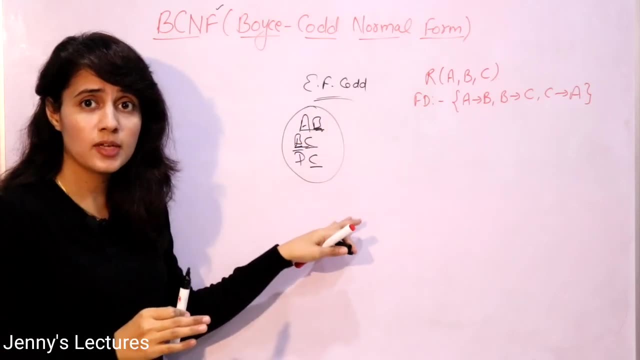 let us discuss that. what are the rules for a relation, what are the requirements for a relation to be in bc nf? and after that we will discuss, with help of two or three examples, that some this, this type of question would be given and you have to tell this as in bc nf or not. 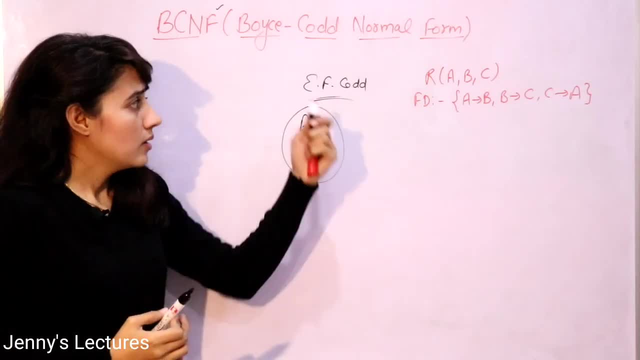 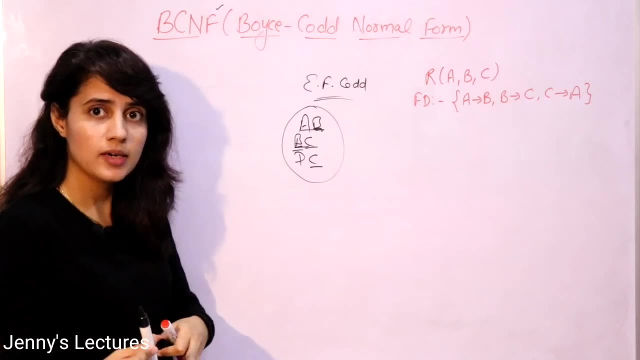 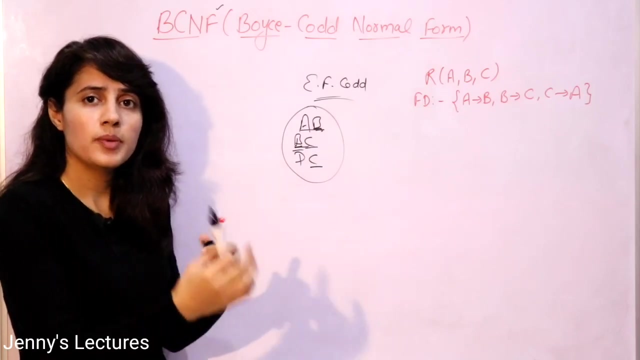 and we will also see with one example that you have to tell the highest normal form exist in that relation, whether it's second, third or bc, nf, right, and after this video we will discuss what is decomposition and after that we will discuss if a particular relation is not in a 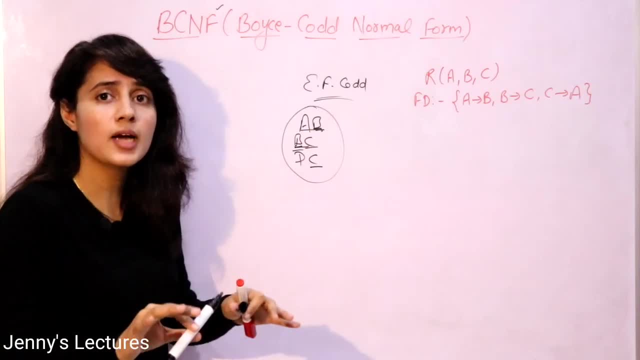 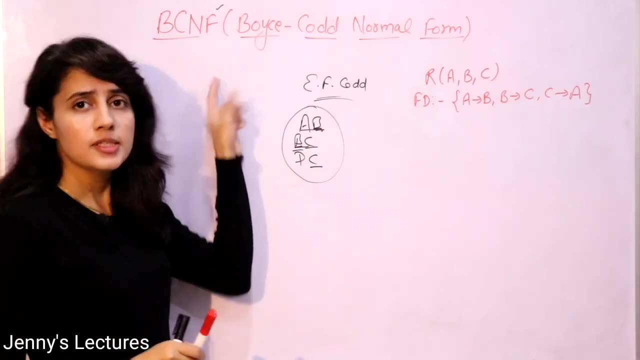 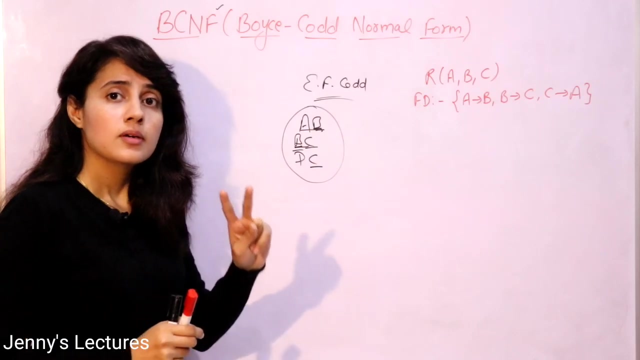 desired normal form, then how to decompose that relation, how to convert that relation into desired normal form. you so the rules are: you can say a relation is in bc nf if- and only first one is- it is in third nf right. second rule is the for each non-trivial functional dependency. see, i'm talking about 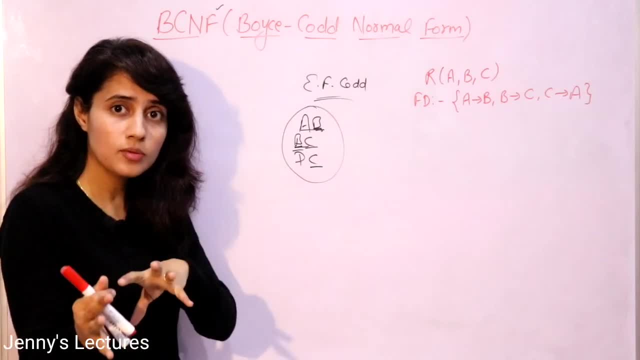 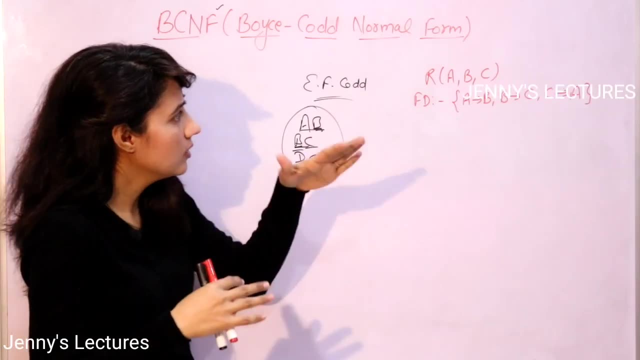 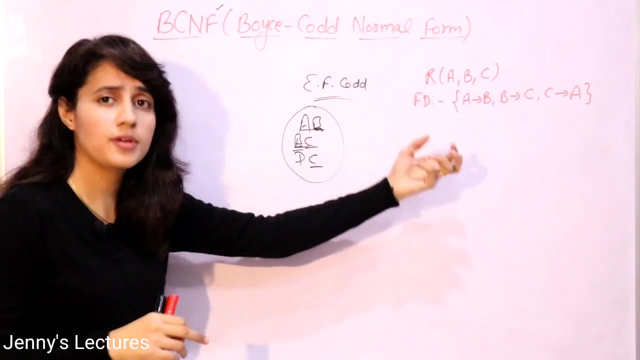 non-trivial functional dependency, not trivial right in the third normal form. also, we have discussed the rules on non-trivial functional dependency right and by default. by default we assume that all the this, this relation given, is in first normal form, plus these dependencies given are in. you can say uh are non-trivial because we we usually take those. 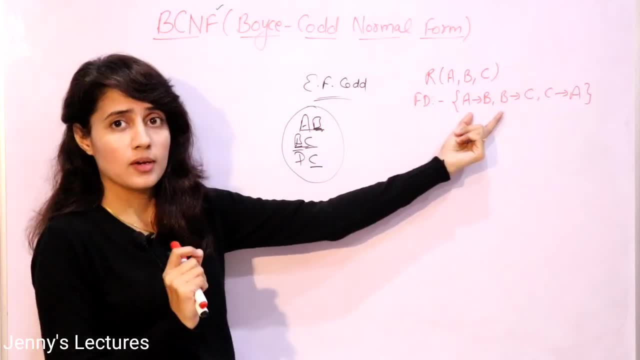 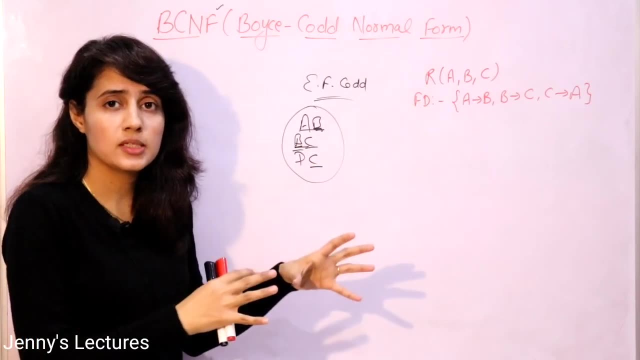 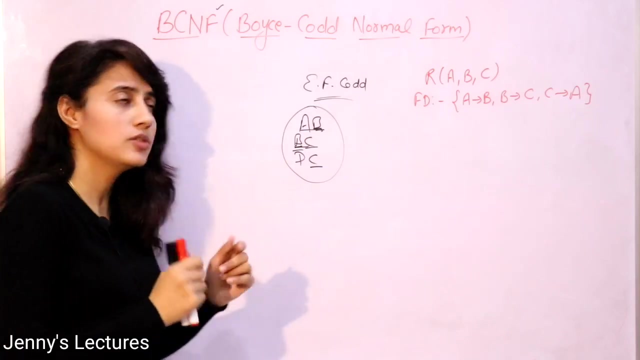 kind of dependencies that are non-trivial, right. so second rule is: for each non-trivial functional dependency, the left hand side of the dependency must be super key, or you can say the determinant must be super key. let me write down these rules. so these are two rules. it is in third nf. second: 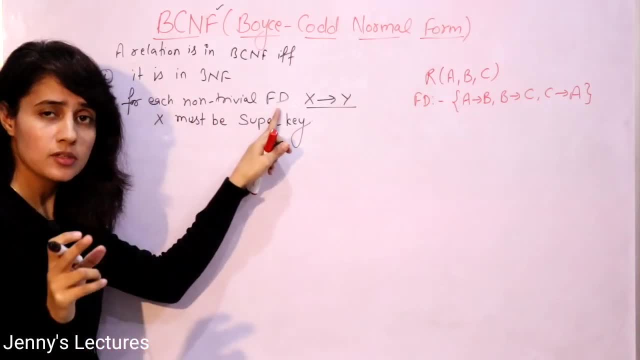 is this one for e-nf and this one is in third nf and this one is in third nf, so this one is in first. each non-trivial functional dependency. I have discussed what is trivial, what is non-trivial functional dependency. suppose functional dependency is x to y right, then x the left. 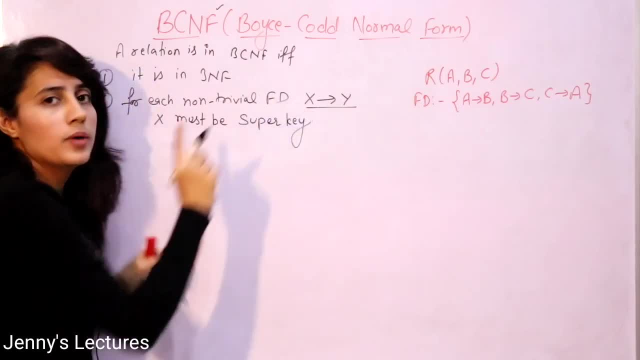 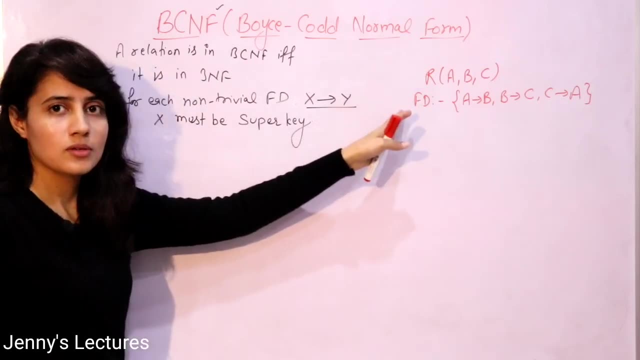 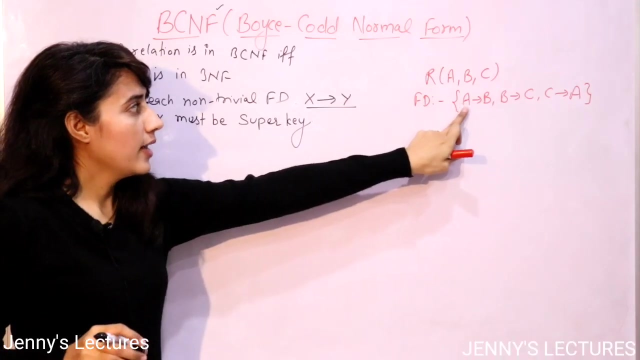 hand side of the dependency must be super key. so it is very easy to check if a particular relation is in b, c and f or not. just you have to find out the super keys. or if you don't want to find out all the super keys, then you can go for each dependency and you can check: a is super key or. 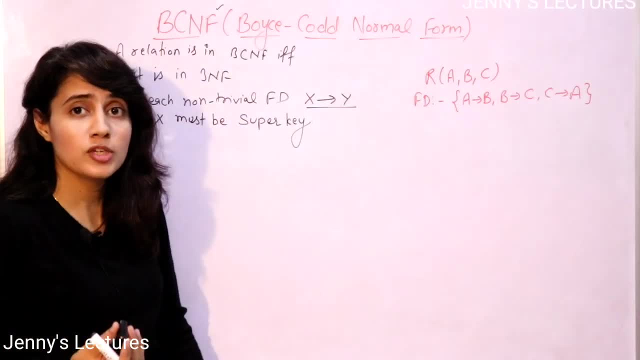 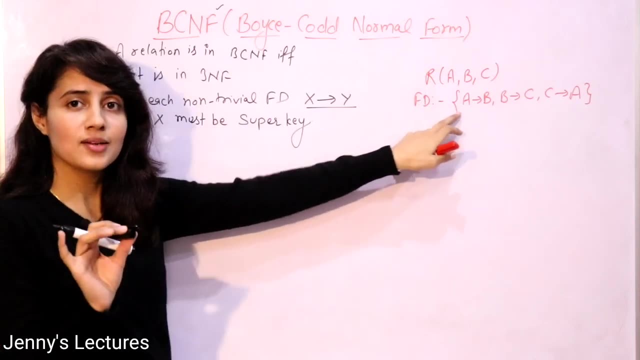 not b is super key or not and c is super key or not. and how to check the particular attribute or particular key is a super key or not? just find out a, find out the closer, attribute closer. and if attribute closer contains all the attributes of a given relation, then that is what a super key. 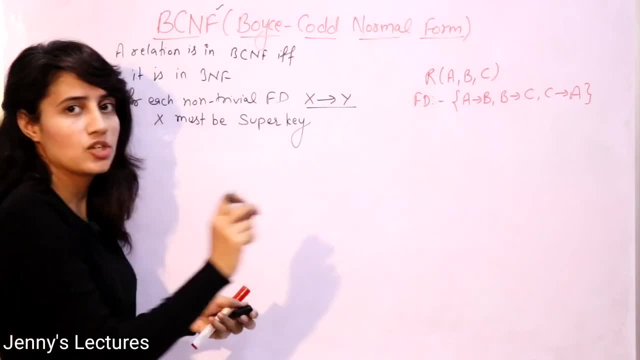 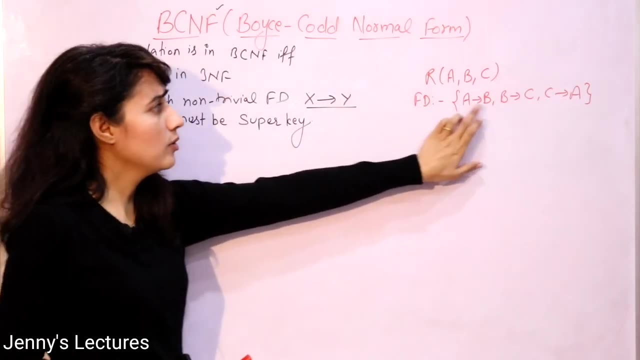 right. so let's check this relation is in b, c and f or not? fine, c. so here I'll not simply check that this is super key or not, this is super key or not, or this is super key or not because, okay, obviously they'll give you these type of questions in gate and net. they'll give you a particular 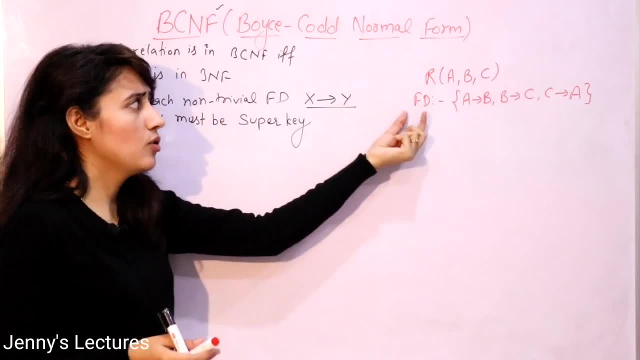 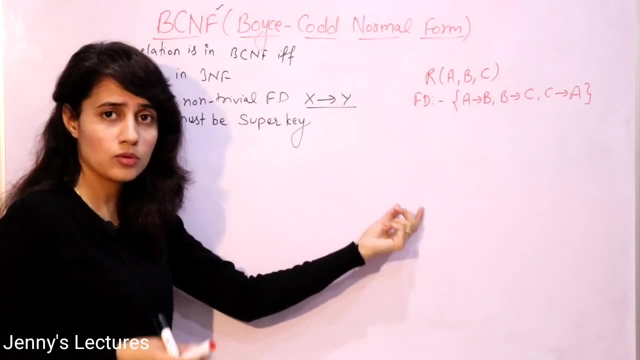 relation, functional dependency, and they'll ask the highest normal form exist in this relation. so for that obviously you need to check, for third also and second also, and for those normal forms you need to find out the candidate keys. so let's find out the candidate keys first. 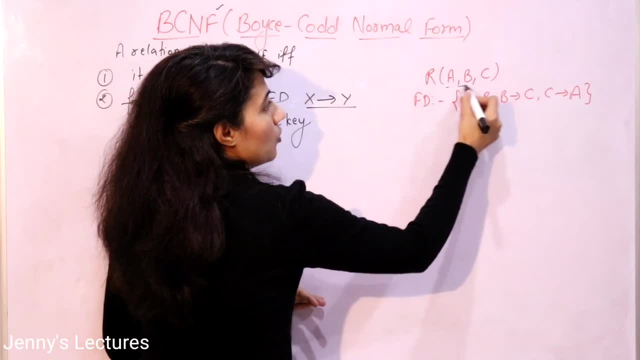 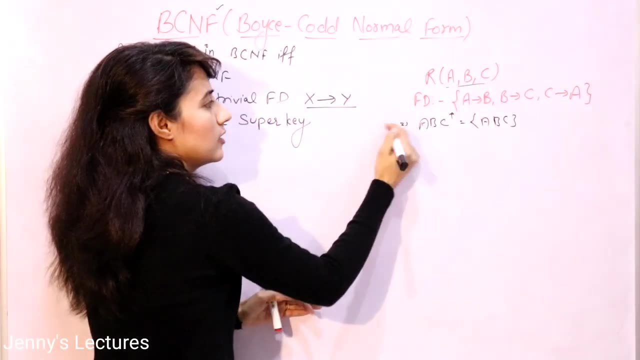 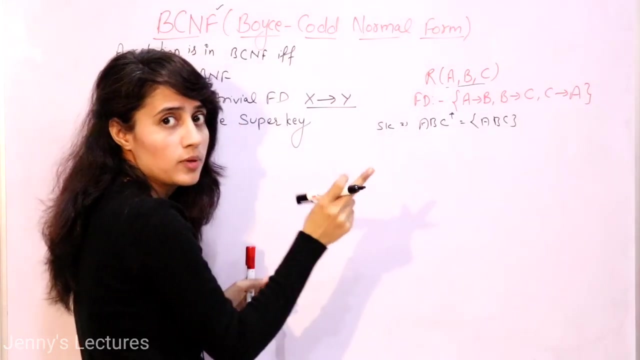 of all. after that we will check how to find out candidate keys. see, take the all attributes, take the closer, and definitely that would find out all the attribute of the relation, so you can say that this is a super key. now find out candidate keys. you discard as many elements, as many attributes as you can, because 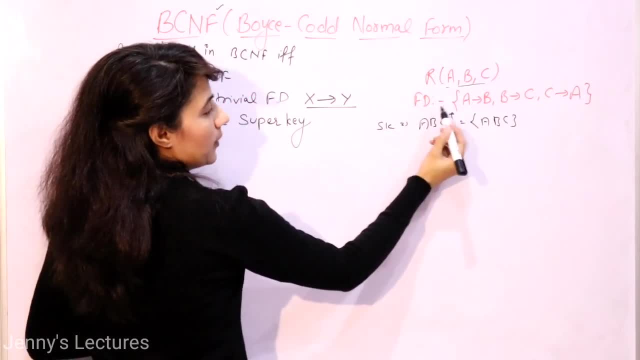 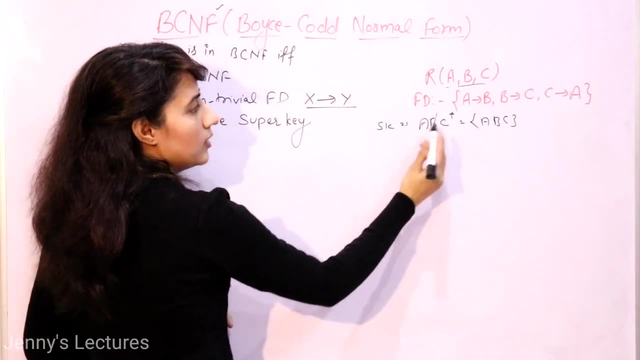 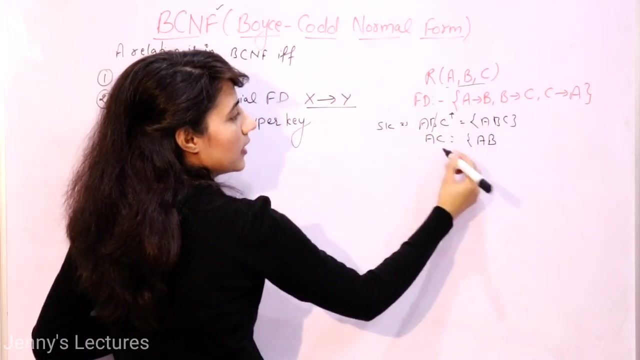 candidate key is what a minimal super key? check out the functional dependencies. how to discard? check out functional dependencies? see a, determine b. it means I have a so I can discard b, because using a, I can determine a and as well as, if you have a, you can determine b right and it will. 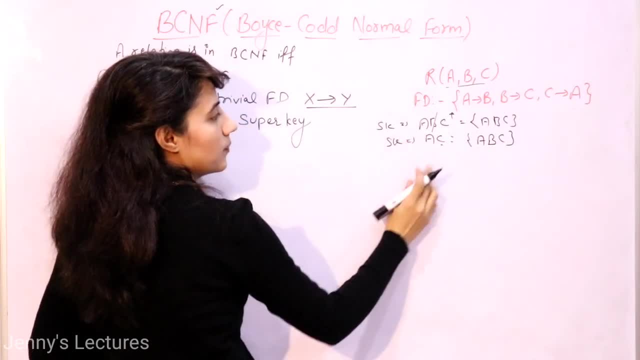 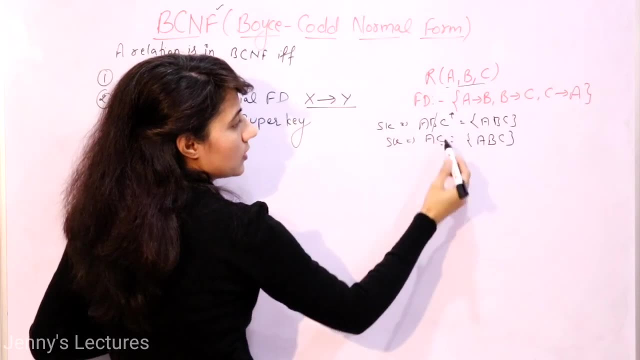 determine c, it is still having all the attributes. so this is what still a super key. now can you discard anything else. a determine b, b determine c. it means a will determine c by transitivity property, so you can discard c. so here I am left with only a. now a is what super key? obviously. 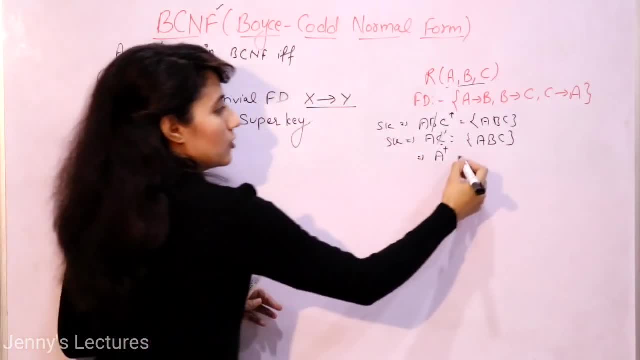 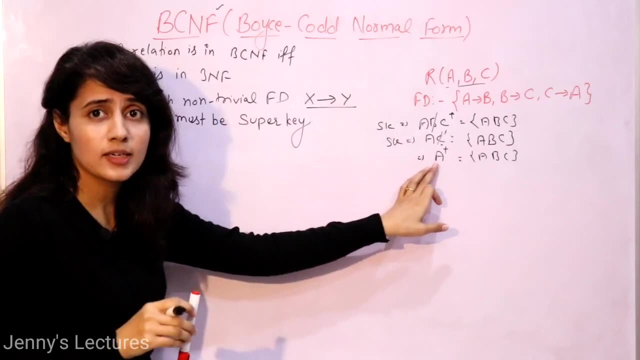 we will. we are not going to discard anything else because it is single attribute. single attribute, this will attribute closer, will contain all the attributes. so it is super key. now check it as candidate key or not. definitely it would be candidate key. why? because it is containing a. 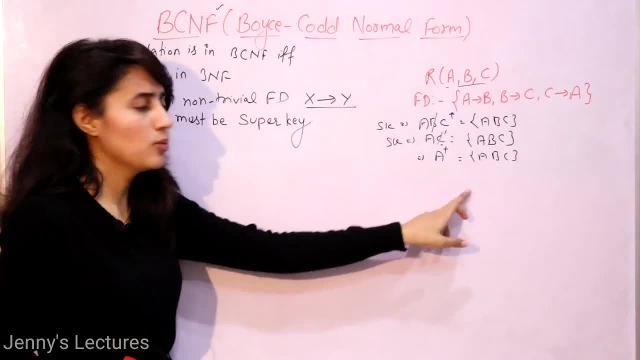 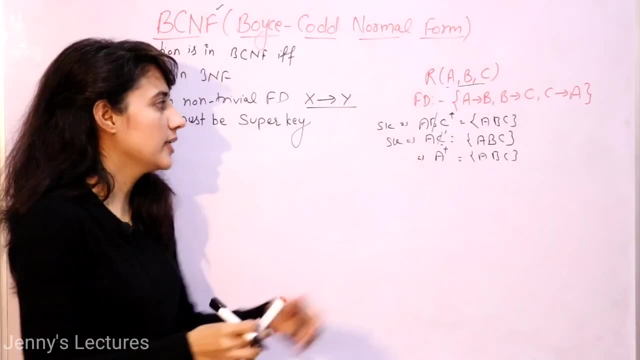 single attribute and no proper subset would be possible. if no proper subset is possible, there is no chance that the proper subset of this would be a super key. so that is why it is a candidate key. so if a is candidate key, then prime attributes we got a now have. 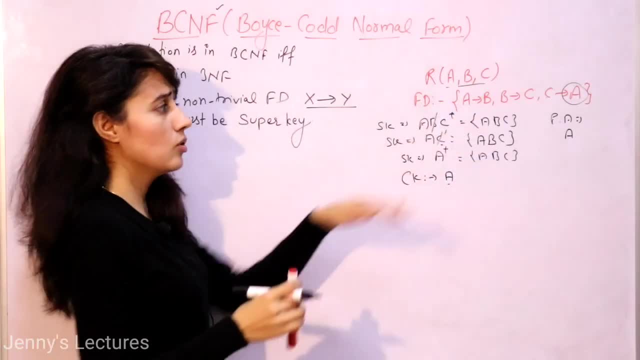 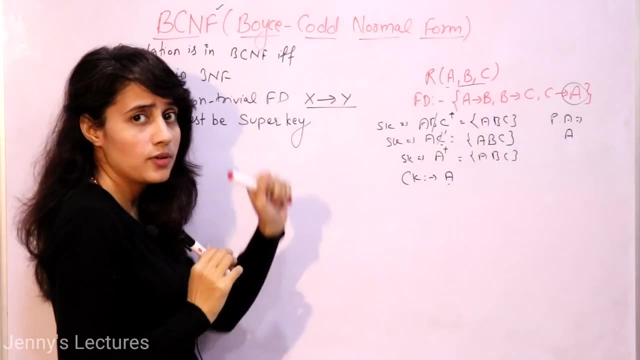 to check that still more candidate keys are present in this relation or not, if prime attributes are present on the right hand side of any functional dependency. I have already discussed this trick in the previous video. you can check out that video in the side button. then there would be more candidate keys. so check out: prime attribute is a- is a present on the right hand? 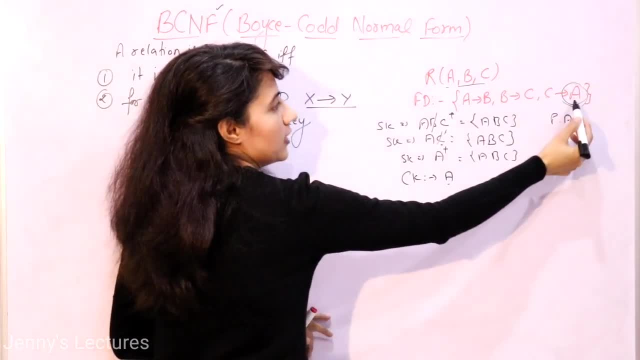 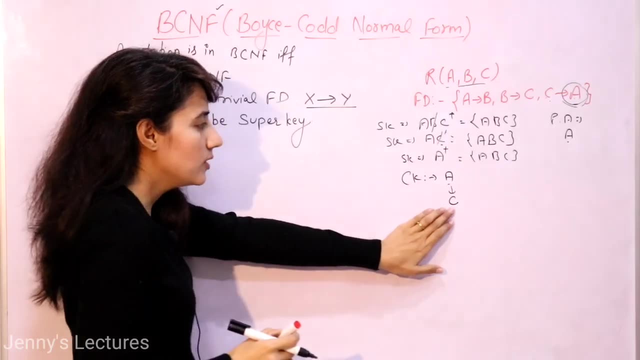 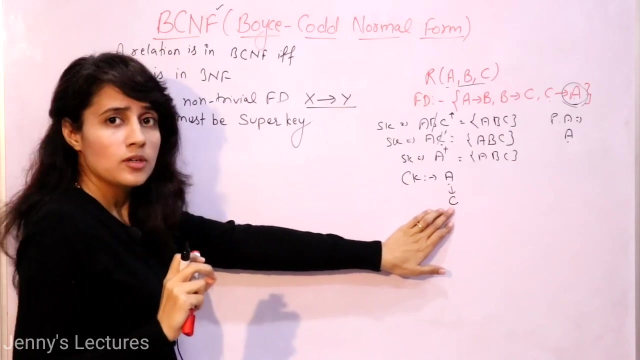 side of any functional dependency. yes here, so you can replace this a with c in candidate key. candidate key is a, so you can replace it with c, but we cannot say that still it is a candidate key. you have to find it out. it is super key that thing. I can definitely see now how to check proper subset of c is possible. no, so if 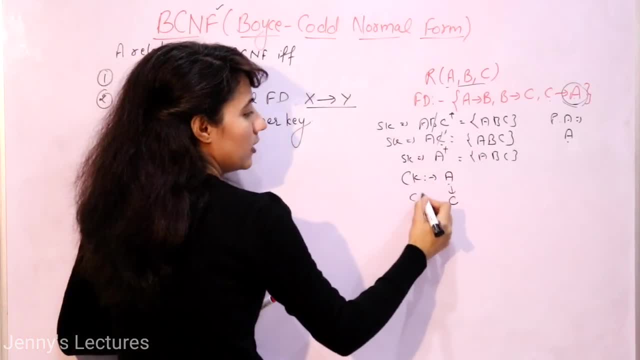 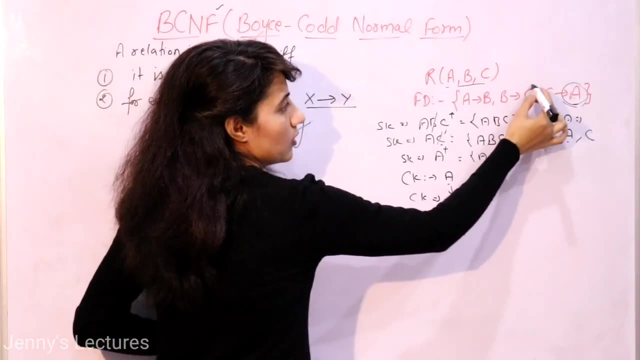 no proper subset is there, then definitely that would be candidate key. so we got two candidate key, a and c, prime attribute, a and c. check again: c is now prime attribute. now c is present on the right hand side of this functional dependency, so we can replace this a with c in candidate key. so we 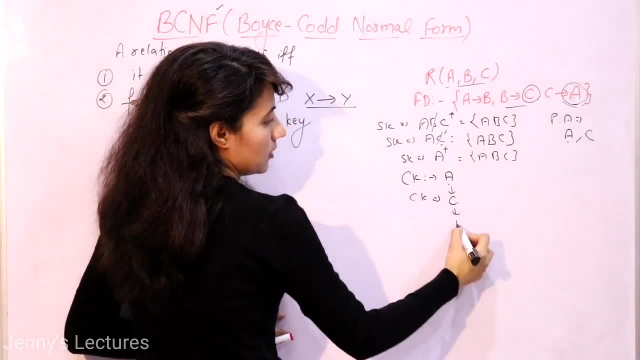 can replace it with c as well. now we can check one more time: Nacht ofタ ind oranges, let's say, now we can check that medicinal hunting circle. so we, you can get this last one and you can look for a few ways to. Ko can get this one and you can, like you can. 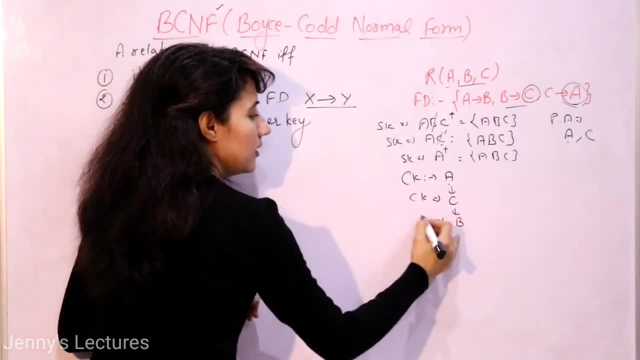 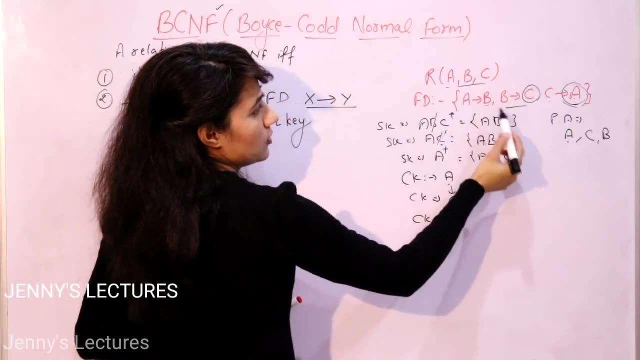 directly see both of them by quickly looking at both of them and you just immediately recognize the two sub-oby備 categories. word isn't it double? 3, two c, one is being right a, two characters. so we have set them right. no b, one is now. it's printed in. 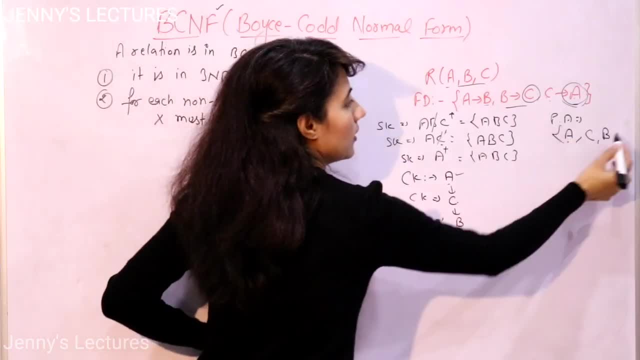 fibre. for last, it is yep b. one is here. so, if we look carefully, are these 3 keys? are protein? is the same list back? it is single attribute. yes, so we can move this. died here after all. that was all right. let's see now what is the? also a and bischen. the one is: 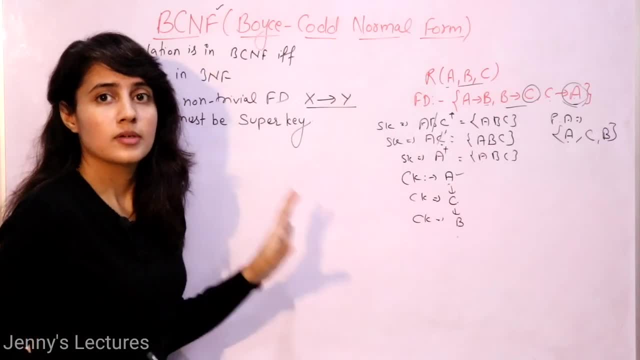 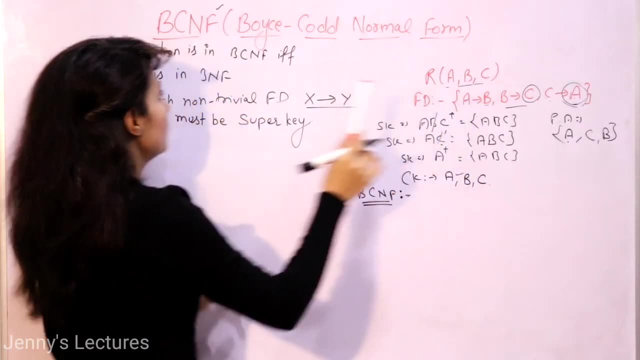 a and c prime attribute are the one that looks all right. so now we have this blank and we can chegarly see all the attributes are prime attributes. now you check this is in BCNF or not. now check for each dependency. see: first of all, it is in third NF, it should be in third NF. so this: 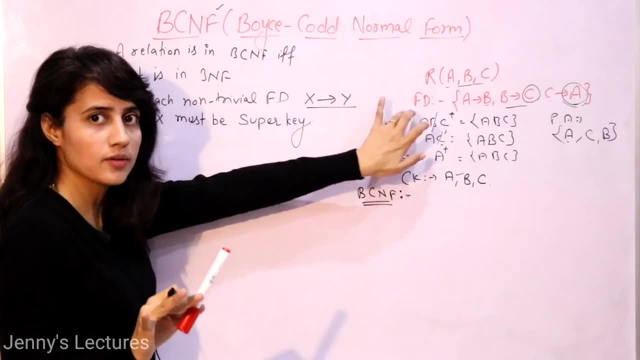 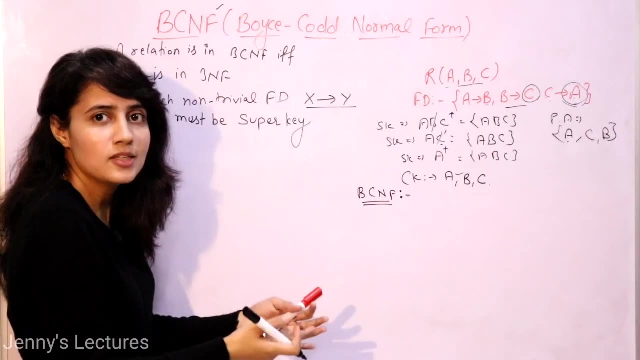 is in third NF. I have taken this kind of example that it is already in third NF, right, and if you want to check, then you can check. there would be no transitive dependency because all the attributes are prime attributes and transitive dependency is what known prime. 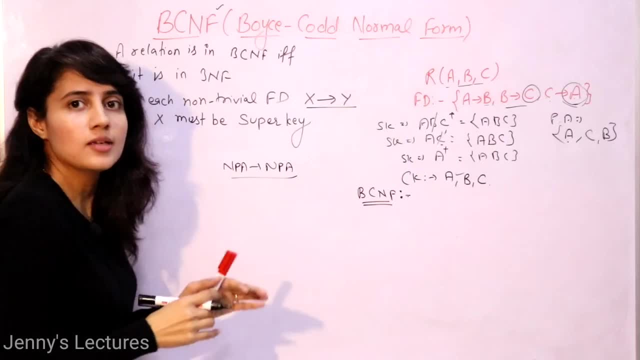 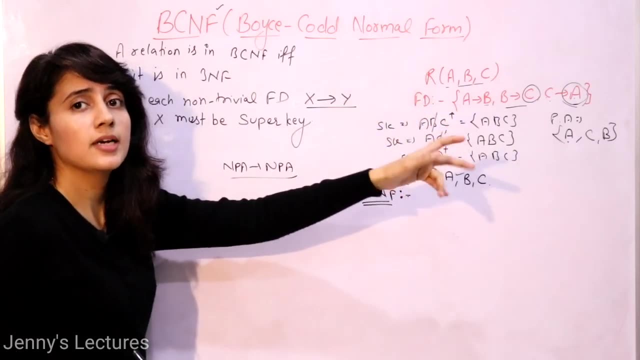 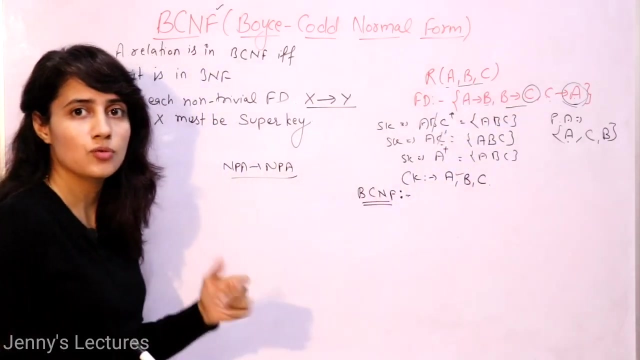 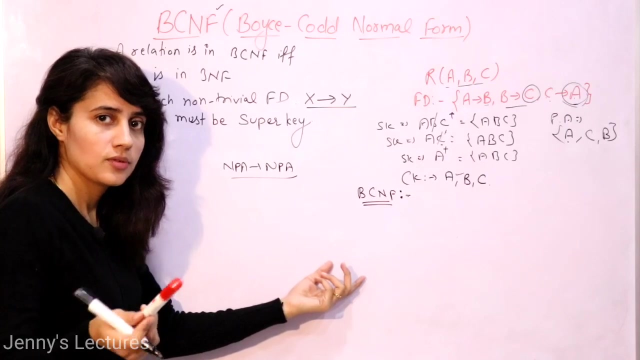 attribute, determining known prime attribute right or another. in another words, you can say: first, either left hand side is super key or right hand side is prime attribute right. if any of these 2 condition holds each functional dependency, you can say that this. then you can say that there is no transitive dependency and that relation is in third NF right now. 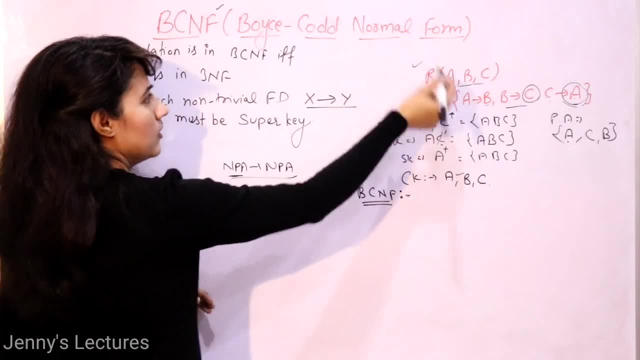 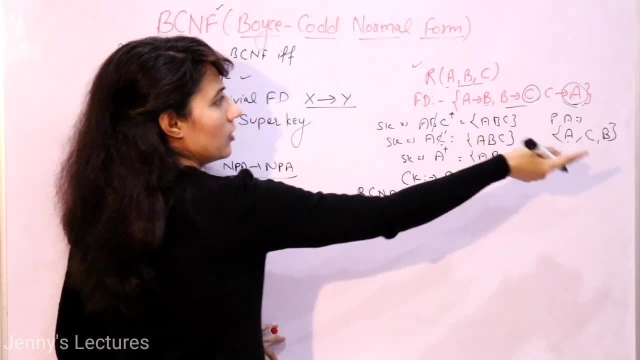 there would be no known prime attributes because all are prime. so that would definitely be be in third NF. Check for BCNF. This is true Now for each non-trivial functional dependency. these three are non-trivial functional dependency. X must be super key. Check this left hand side. 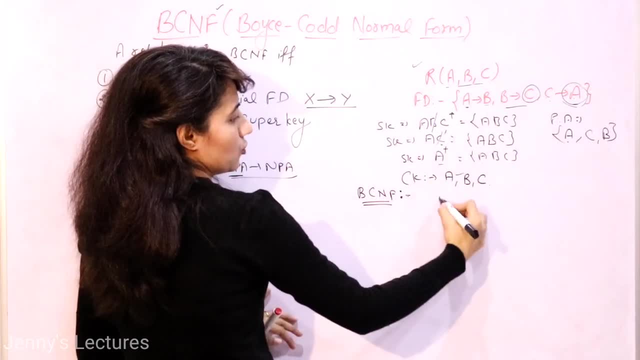 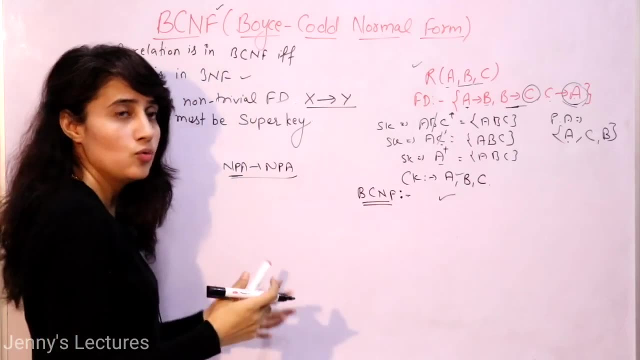 must be super key. Is A super key? Yes, So first is what? According to first, it is in BCNF. Now check this: is violating the rule of BCNF or not. Is B super key? Yes, B is candidate key, Definitely. 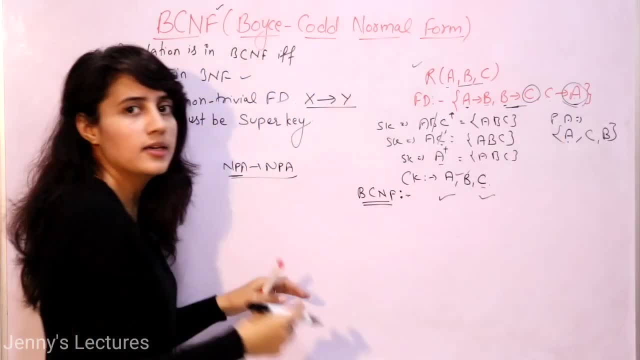 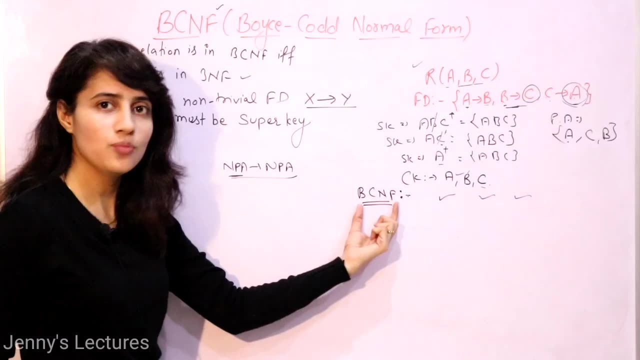 it would be super key. Yes, Is C super key? C is candidate key. Definitely it is a super key. So yes Means each functional dependency is satisfying the requirement of BCNF. Right, So you can say that this relation is in BCNF. See why we are saying that it is more strict. 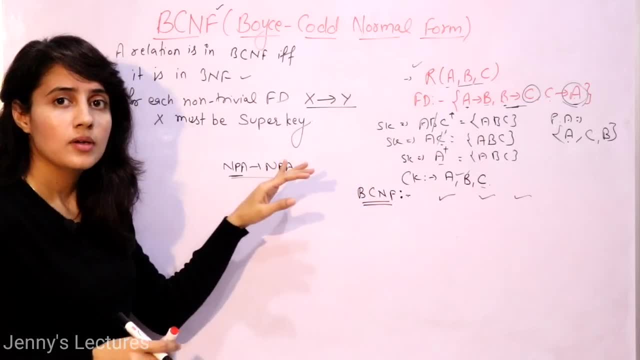 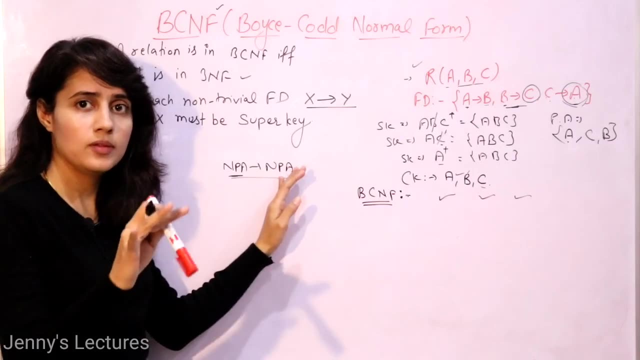 than third NF, because in third NF we have what rules? Either left hand side is super key or right hand side is prime attribute, Then fine, that would be in third NF, Right. But here we have a rule that is not in BCNF. So we have a rule that is not in BCNF. So we have a rule. 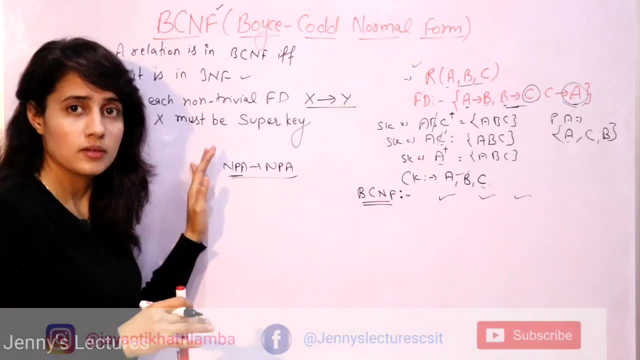 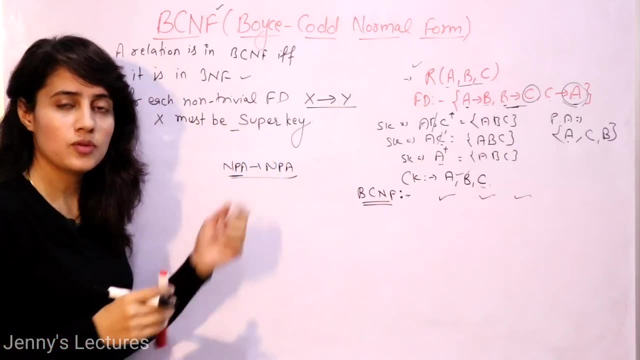 that is not in BCNF. So here definitely the left hand side. you can say the left hand side must be super key, Right? No other condition is there. This must be satisfied. So that is why we are saying that it is a, you can say, more strict version of 3NF, because 3NF doesn't deal these. 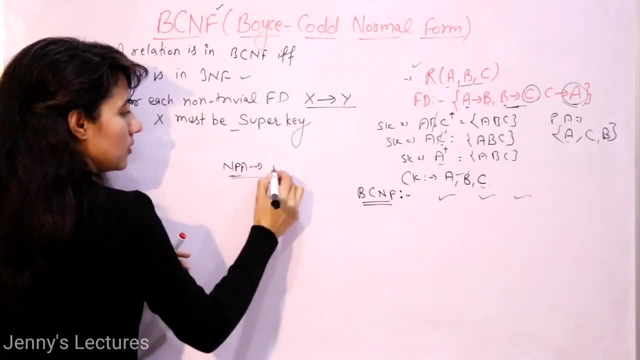 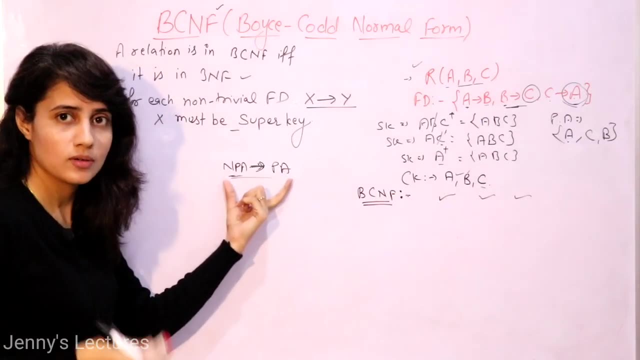 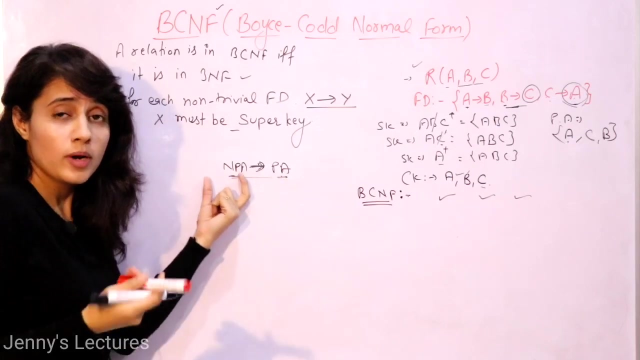 kind of conditions Like: if a known prime attribute is determining a prime attribute, then according to third NF it is not a transitive dependency. Why so? Because right hand side is prime attribute, So it is not going to deal these kind of cases. A known prime- 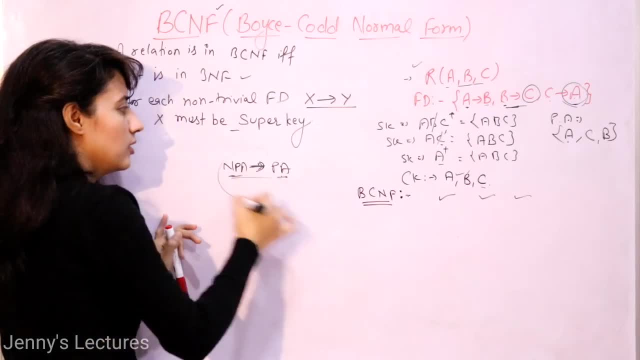 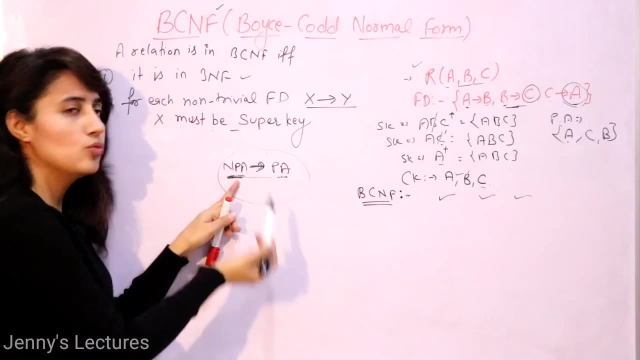 attribute is determining a prime attribute. Because of this dependency there would be some problem, Right? But here, in this case, this left hand side must be super key, But here it is not a super key. So it will not allow these kind of dependency here, Right? And what about second? 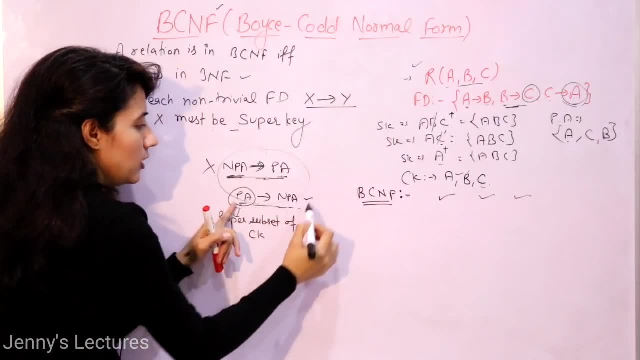 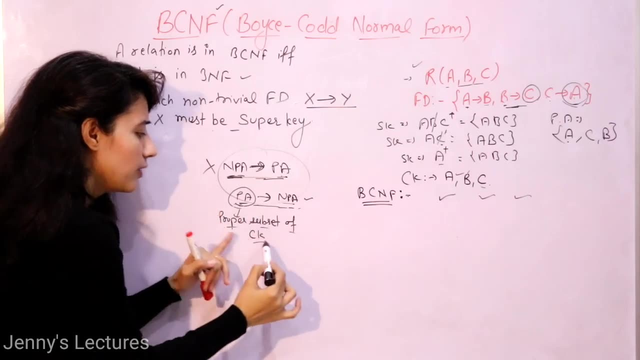 normal form. This will this second normal form deal with these type of cases? Right, If prime attribute is determining a non prime attribute, See prime attribute is determining a non prime attribute means it should be a proper subset of candidate key. It is not like that. it is a proper. 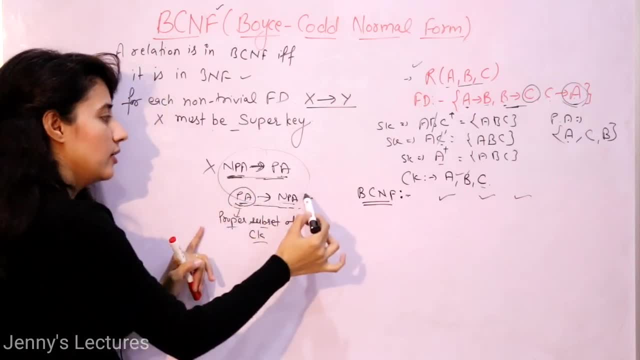 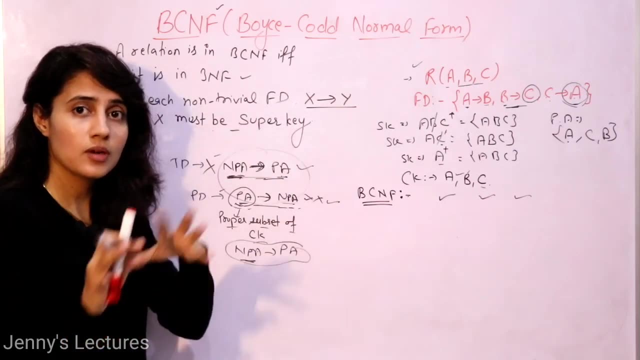 candidate key. It should be a proper subset of candidate key. Then it will violate the condition of second NF, Right? So now you have the idea of all the normal forms: First, second, third, BCNF. Now I will discuss with one example, and I will give you one example and we will discuss that. 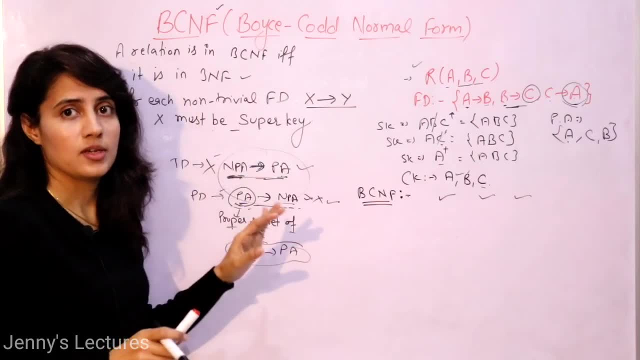 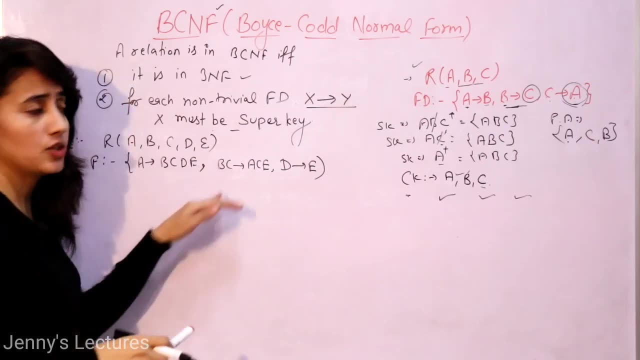 what is the highest normal form given in that relation Right See? Let us take this example and find out the highest normal form of this relation See. So for this, first of all, we need to find out the candidate keys, All the candidate keys. How? 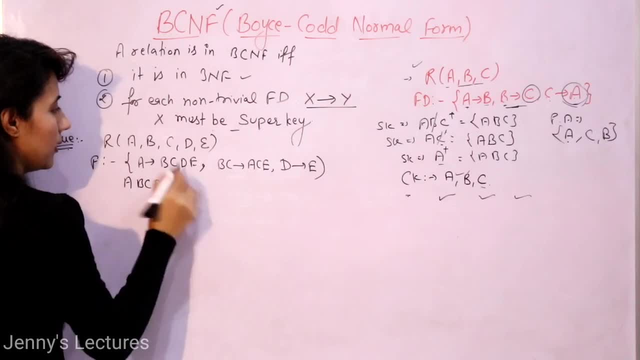 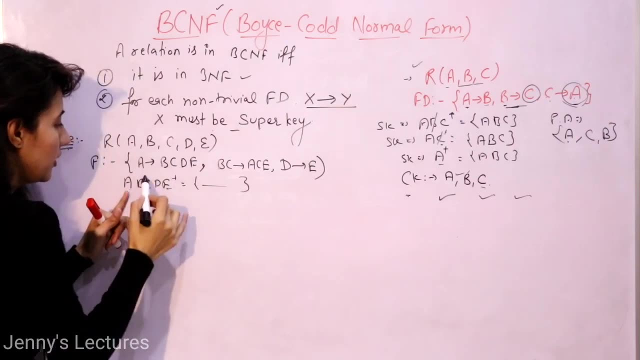 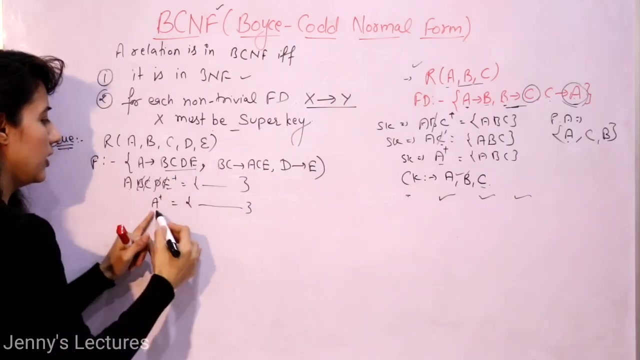 to find out candidate keys, First of all, take all the attributes of this relation Closer. obviously will contain all the attributes, So this is super key. Now try to discard. A is determining BCDE, So I have A. So using A, I can determine A itself plus BCDE using this dependency, So A attribute. 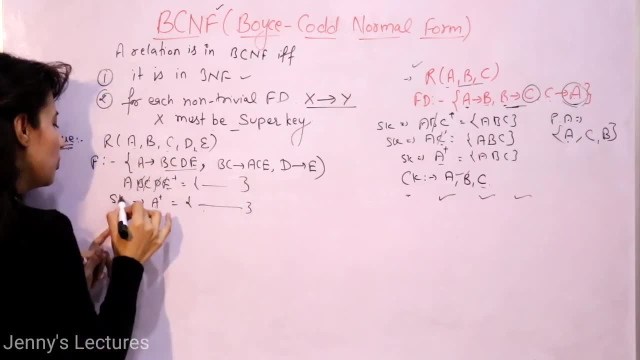 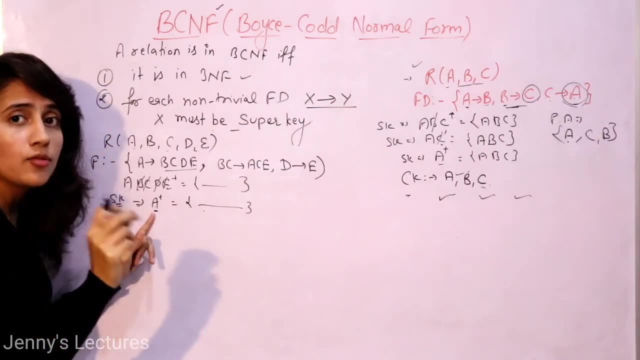 closer of A will contain all the attributes of the relation. So A is definitely a super key. Now A is super key. I can determine A itself, So I have A. So I can determine A itself, So I can cannot discard anything else because it is now a single attribute Right Now. definitely that would. 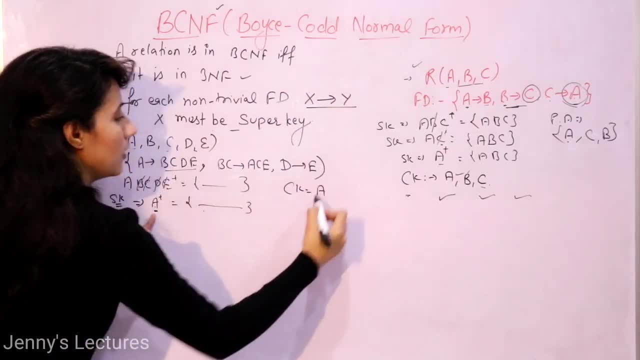 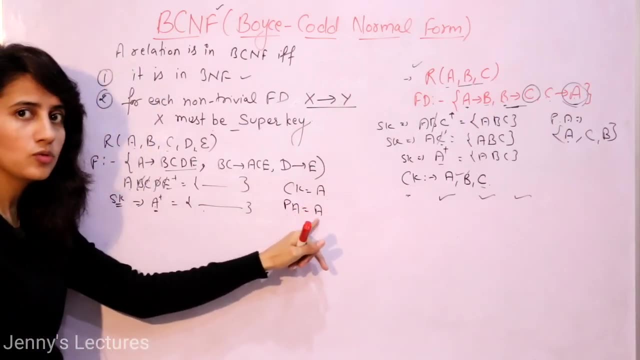 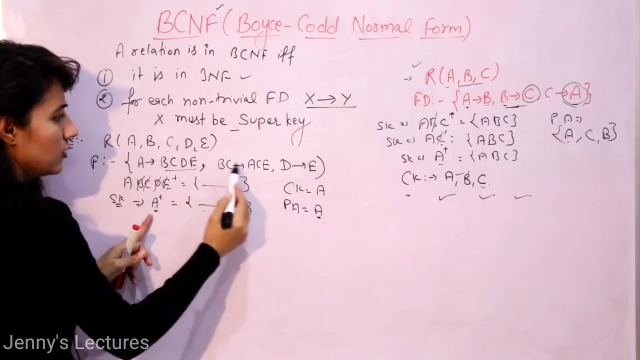 be a candidate key. So now candidate keys are, first of all, A. We got one candidate key Prime attribute. we got A The part of candidate key. Those attributes which are part of candidate key are known as prime attribute. Now check, Is A this prime attribute present on the right hand side of 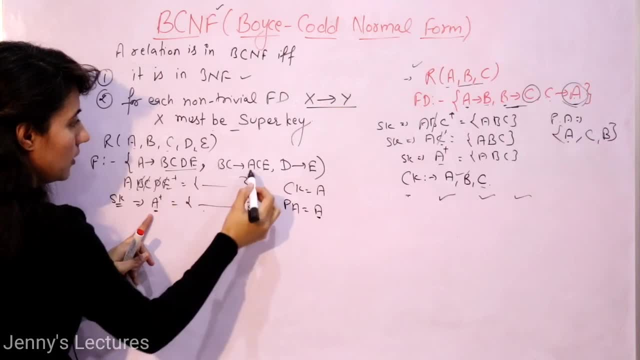 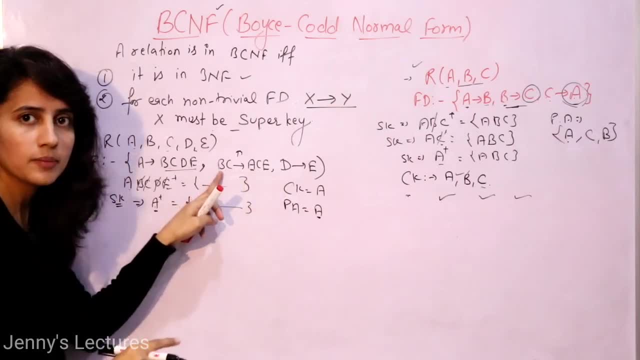 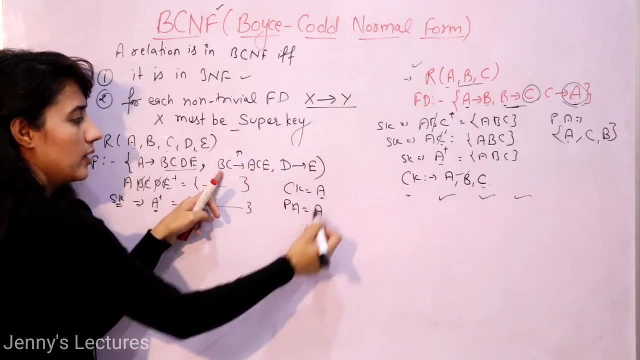 B C determine A. B C determine C. B C determine E Because of that splitting property. So B C determine A. Right, Right hand side we have A. So at the place of A in the existing candidate key I. 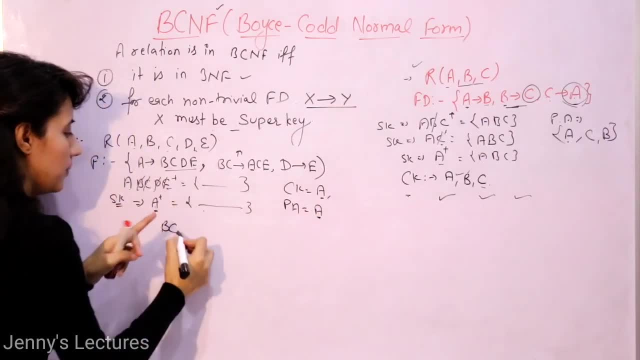 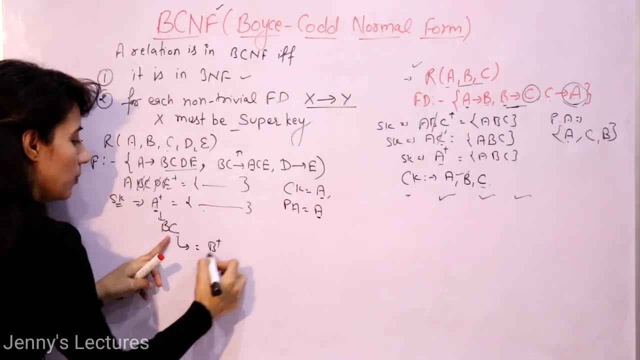 can replace it with B C Right, B C at the place of A, But B C. we cannot say that still as candidate key. You need to check out Now: B is proper subset and C is proper subset. Find out. 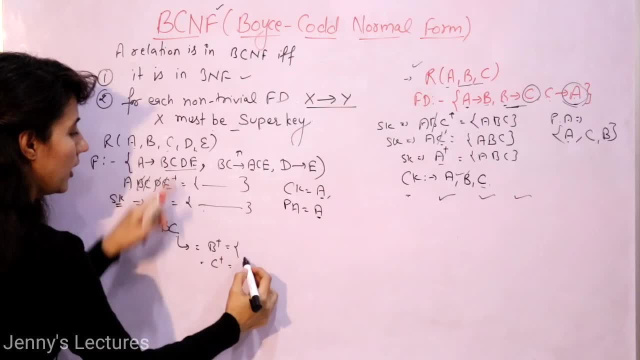 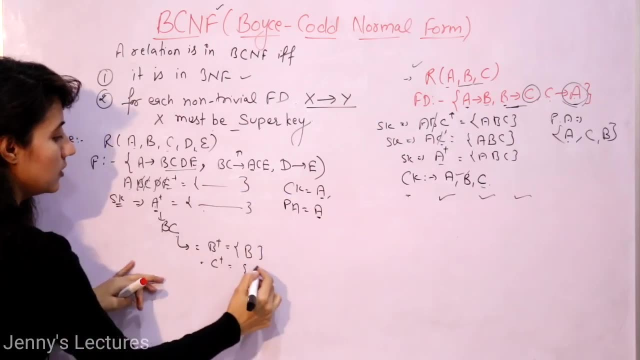 the attribute closer of B and C Is B determining all the attribute. B is determining B, Nothing else, Because here both B, C will determine A C, But we have only B, C is determining only C, Nothing else. So this is not super key, This is not super key. So definitely B, C is what 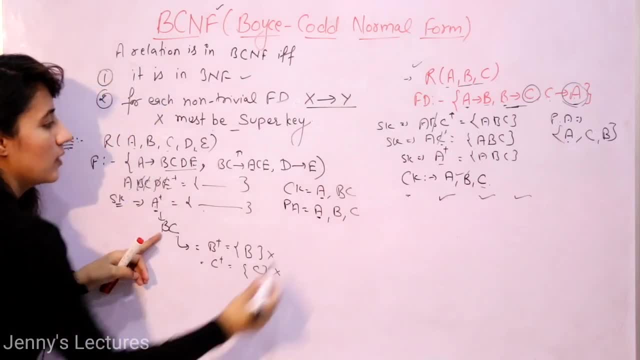 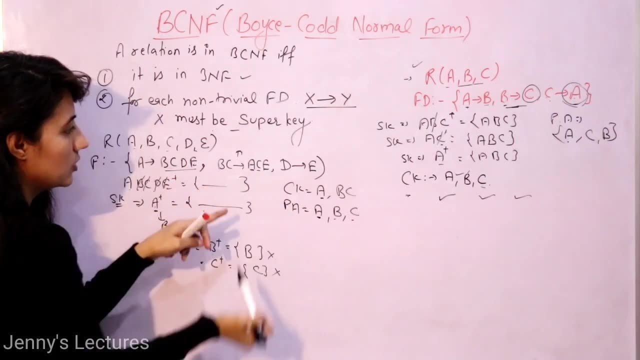 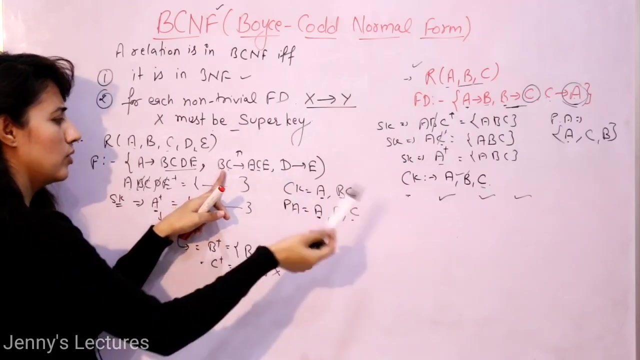 candidate key. Now prime attribute are: one is B, One is C. Now check out: B and C are prime attribute. Those are present on the right hand side of any this dependency or not. Yes, Here we have C Right, But definitely we will replace the C. This is what a trivial functional dependency. So 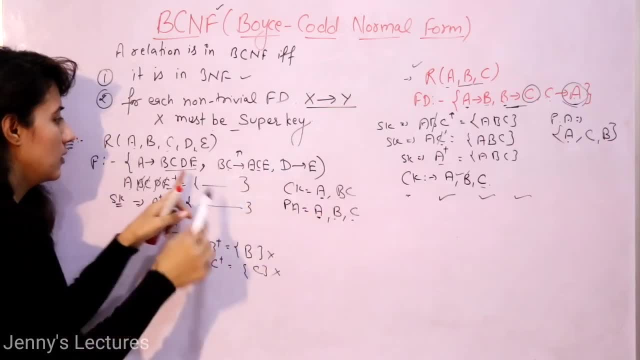 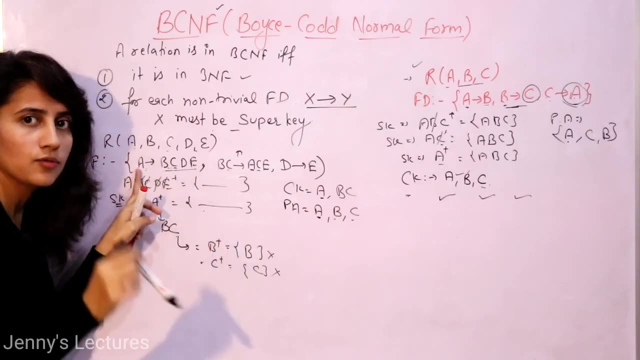 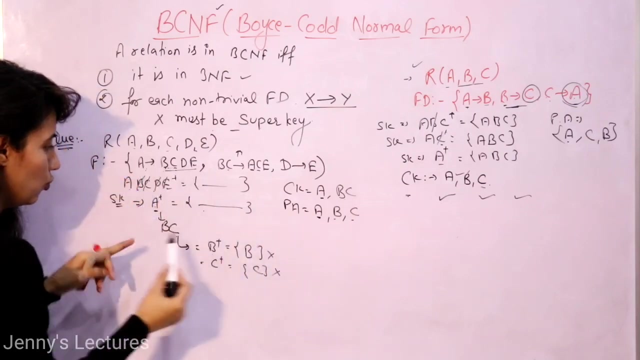 if we replace A with B, C, then that would be same. Right Here we have C. This can be splitted. A will determine B, A will determine C, A will determine D, A will determine E. Four dependencies Right By splitting property Now at the place of B. two cases can be there At the place of B. I am: 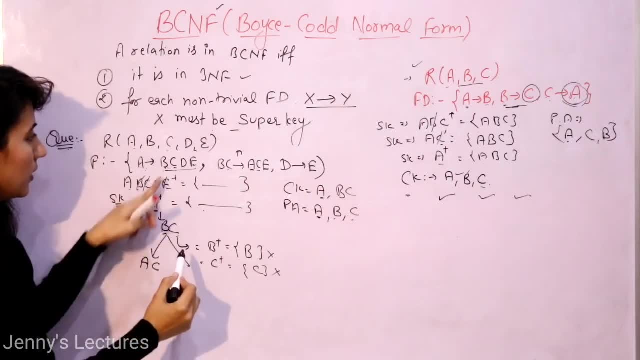 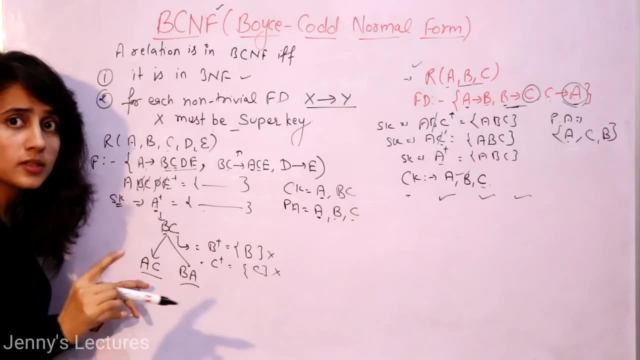 replacing A, So first one, A, C. Now, at the place of C, I am replacing A, So second one is B A. I cannot say that these are candidate keys. Check out, These cannot be candidate keys. Why So? because 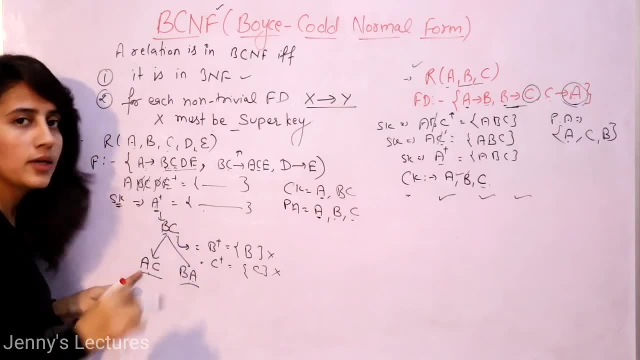 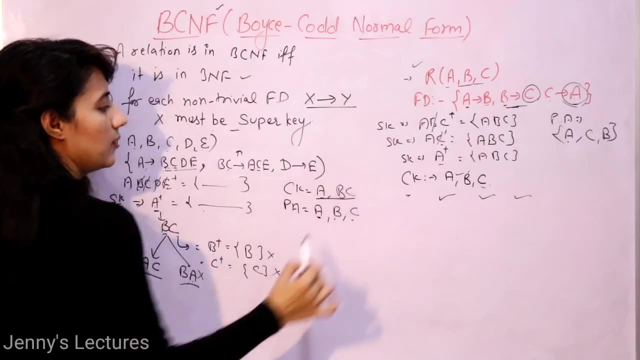 proper subset of this and this is what A and A itself is a super key, So this cannot be candidate key. This cannot be candidate key, Right? So in this case we have only two candidate keys: A and B, C. Three prime attributes are there. Non-prime attributes are D and E. Now check First of all. 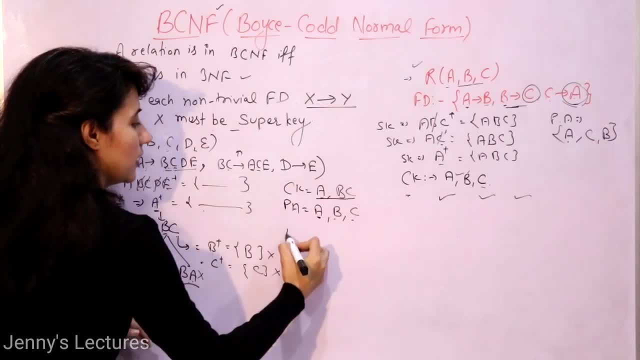 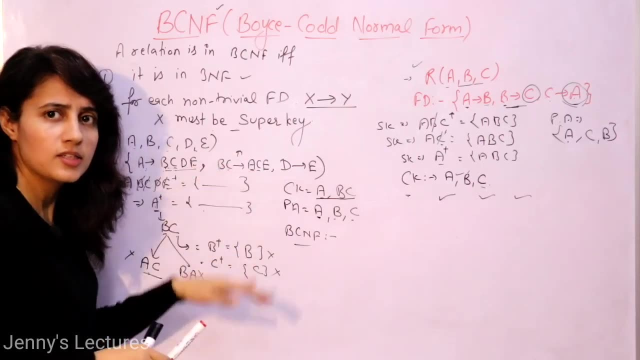 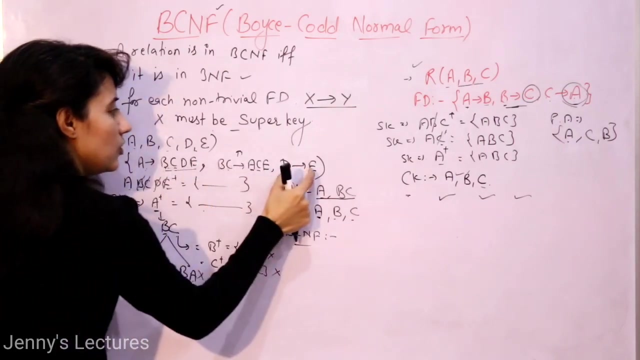 first of all we will check for the highest normal form, that is, for B, C and F. Right, It's better to normal form rather than starting from the second, the lowest normal form, Right, If these type of questions are given. So for each functional dependency we will check the rules. First one is: 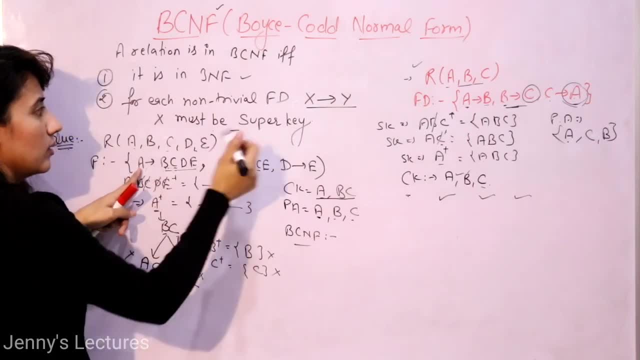 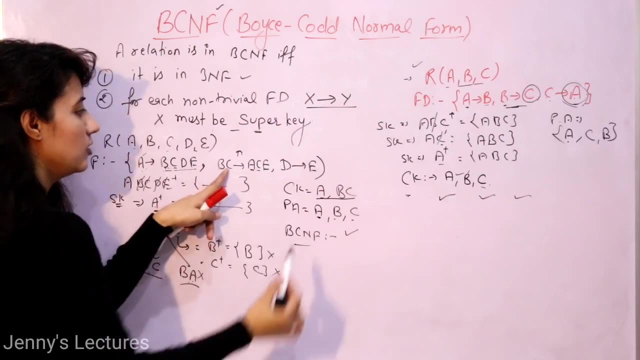 this one: A is super key or not, Because this is the main condition Right. A is super key. Yes, So this is satisfying the B, C and F property. B C is super key. Yes, Because B C is. 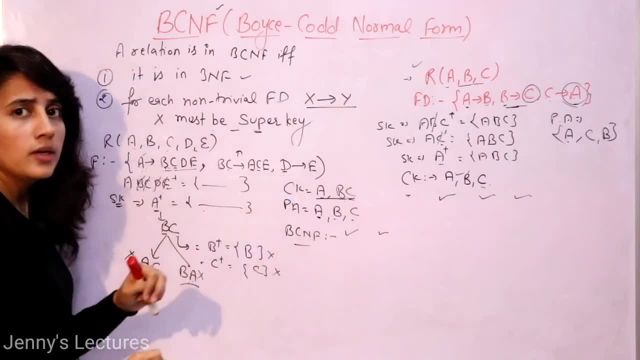 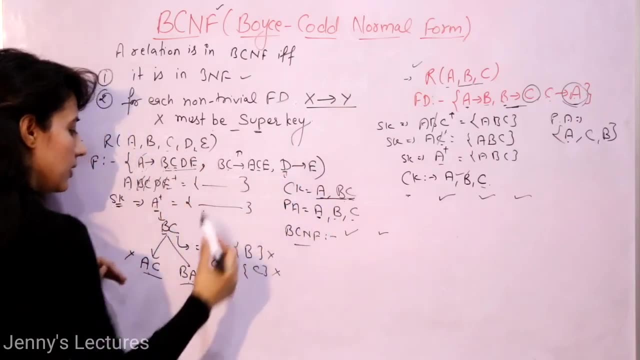 candidate key. definitely it is a super key. Is D a super key? No, Even D is not a prime attribute. And if still you want to check, then you can find out the D closer. If D closer contains all the attributes, then that would be super key. But D closer contains only D and E, Nothing else. 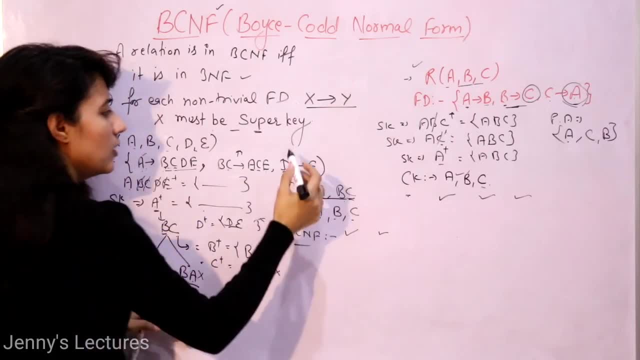 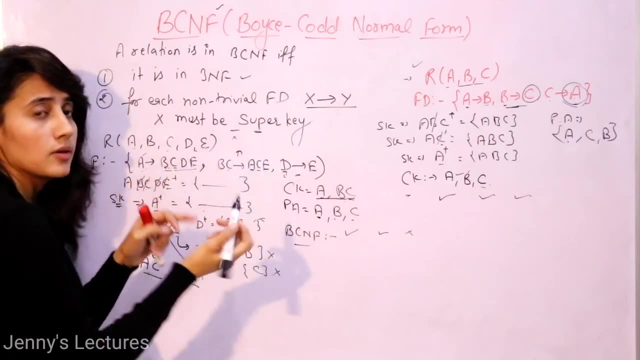 we can derive by D and E, So this is not a super key. So this because of this property. This property is violating the B, C and F rules, So this is not in B, C and F. Now find out. third, 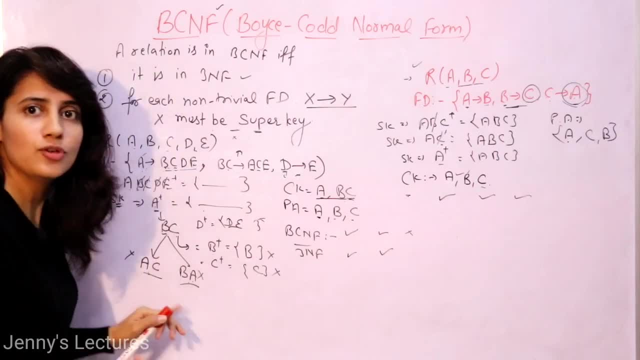 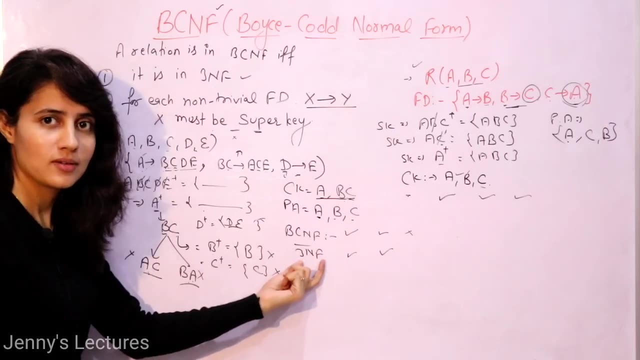 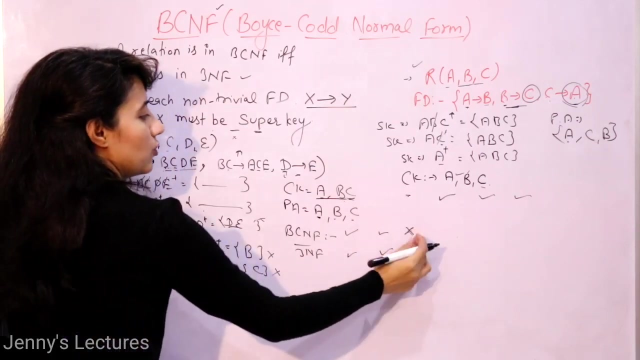 property. Definitely it would be third NF and third NF. No need to check Right, Because for B, C and F that dependency should be in third NF, Right? So that is for sure that D's and D's would satisfy the third NF rules. You just need to check out this one. for this one, D to E Is this: 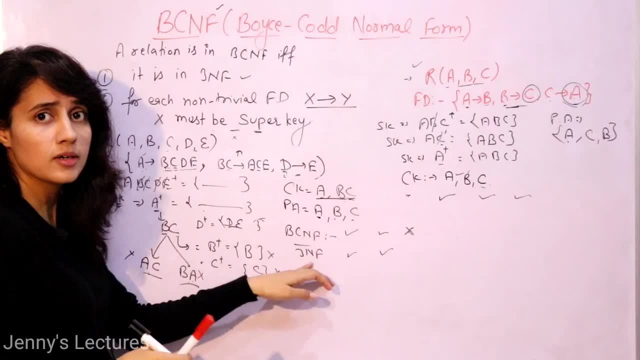 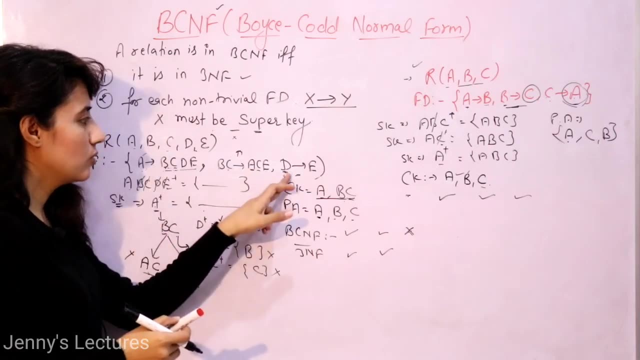 transitive dependency or not, Because third NF, we will check In. third NF, we will check. transitive dependency Means in that case, check out left hand side is what Is super key. No, You cannot say that this is violating third NF. 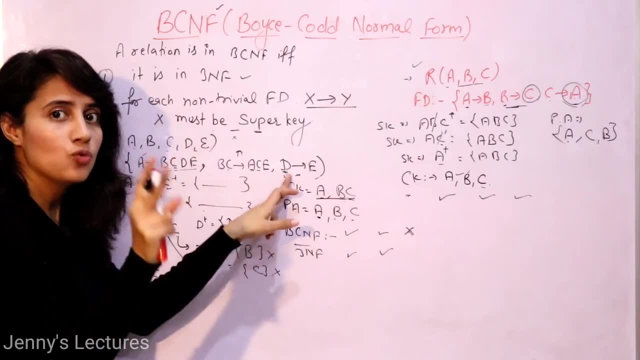 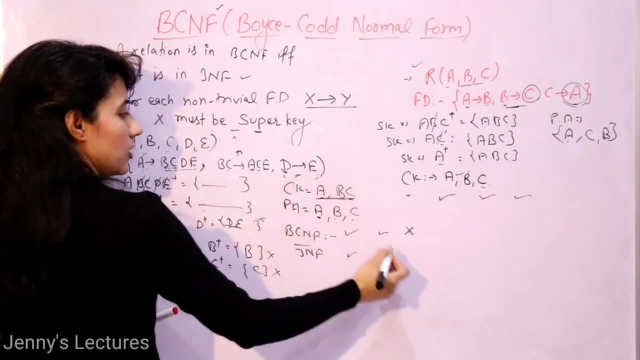 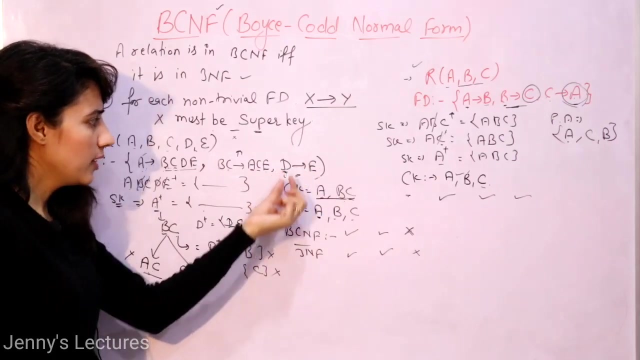 Or right hand side is prime attribute. Two condition: At least one should be satisfied, Not both. So is E prime attribute? No. So now you can say that this is not satisfying. third, NF property. Or in another term you can say: NPA determines NPA, Non prime attribute D is non. 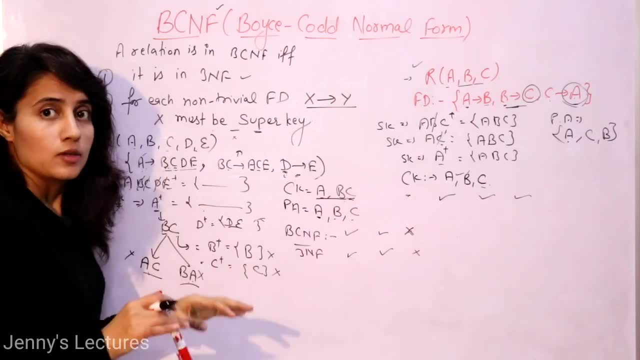 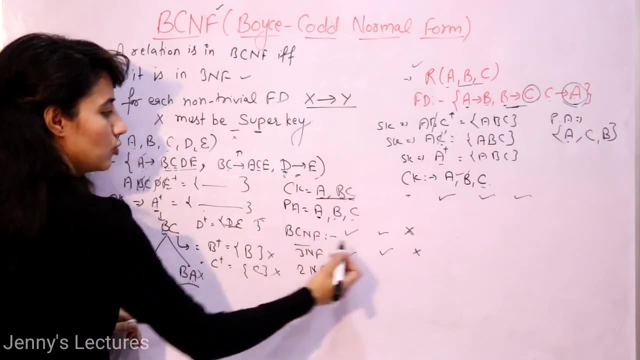 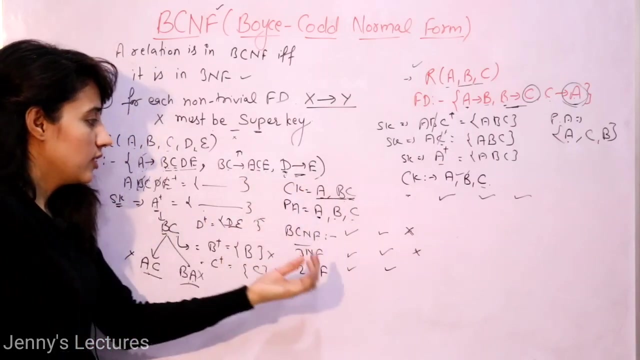 prime attribute: Yes. E is non prime attribute: Yes. So this is transitive dependency. So this is not satisfying the property of F. Now check for second NF: Partial dependency. So this is in third. So definitely in second. Definitely it would be in second. Check out for this one, Right, If you are not satisfied with. 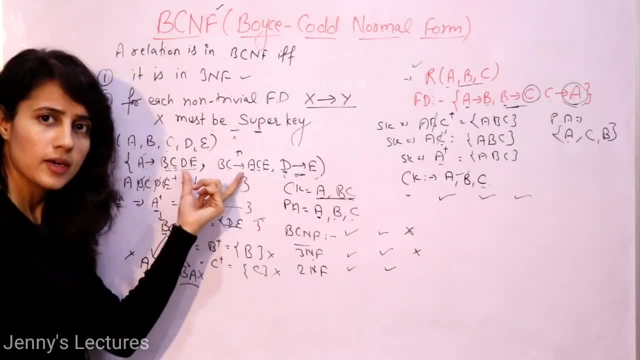 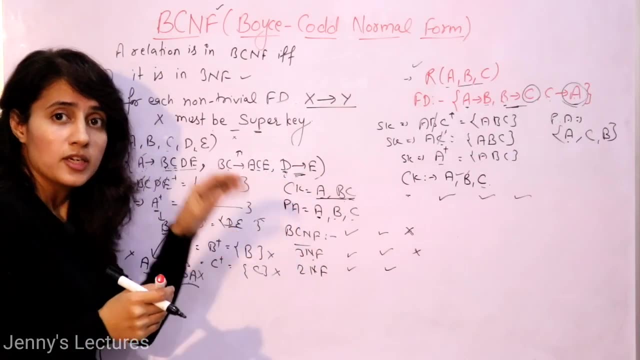 this answer that this would be definitely in second NF, then you can check Right. You will find out that these, this and this- are in second NF. Check out for this one Second NF. we will check for partial dependency. Partial dependency is there. It is not satisfying that property. 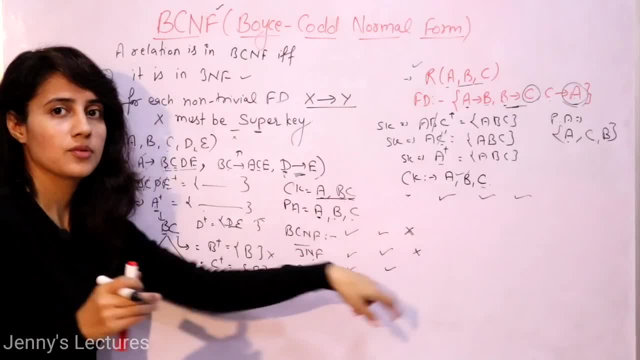 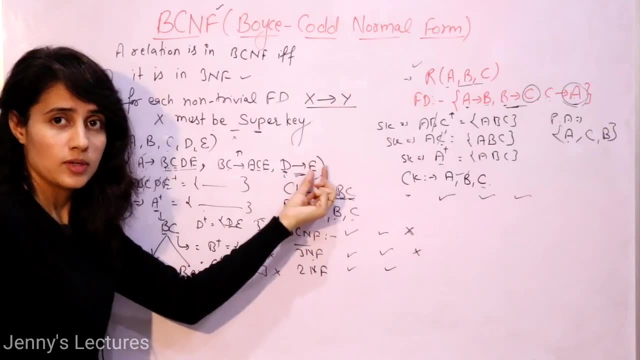 Right, If this is partial dependency, then that is not in second NF. Partial dependency is what This is like. you can replace the colors And this isi of dividing up this in second NF and C and instead I am saying: why not you just try this 0%, you know when you are getting. 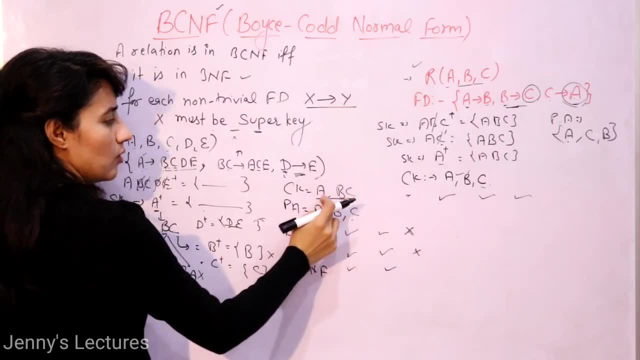 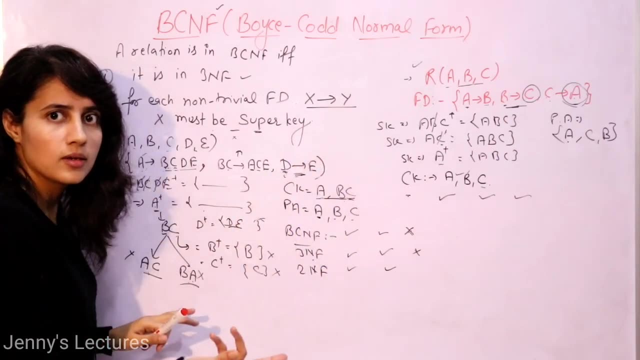 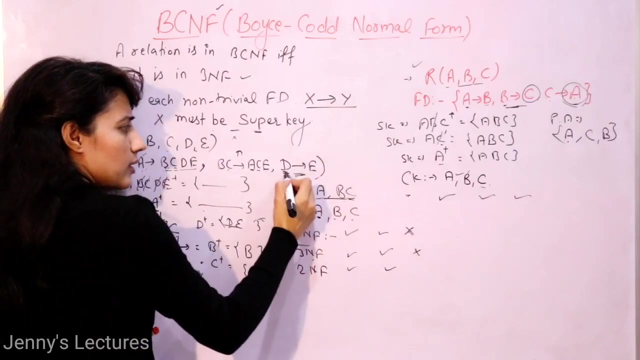 an L ingredients, And here is D supplement. So what will you do? You can, unless you want to run W い, crank it again and run SOOP in the same way. You can purchased the same here and you can come to the next step. Ok, So let us first come look at��� saucer Break. 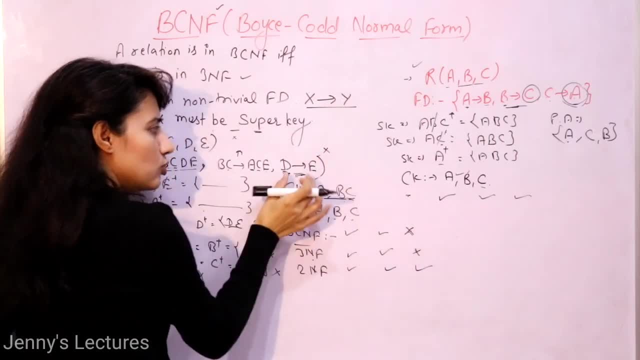 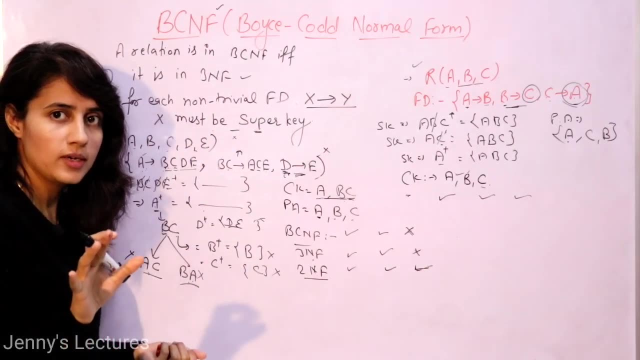 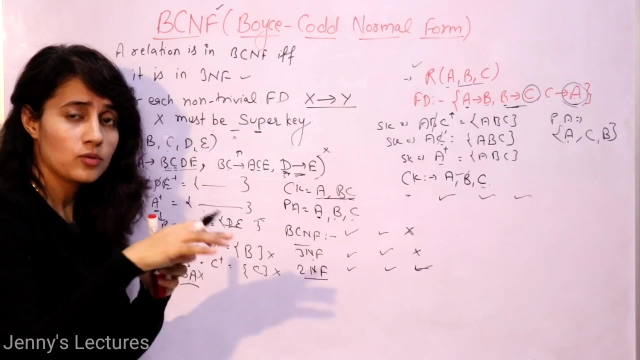 into soy gate partial dependency? if it is not partial dependency, then you can say that it is in second normal form. I hope you are getting my point right. for this video you must check out the first, second, third normal form videos, so you can check out those videos. in the description box I'll provide you the 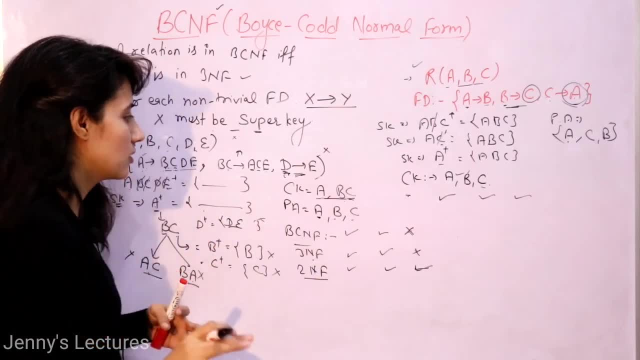 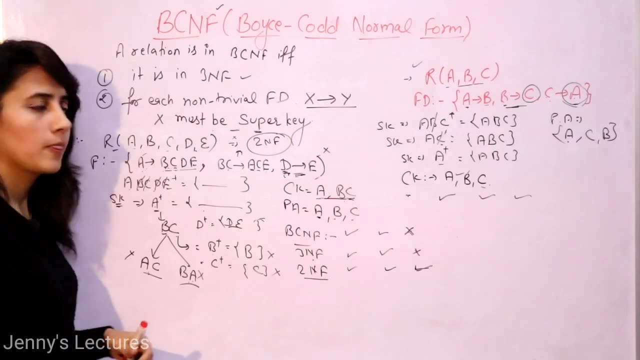 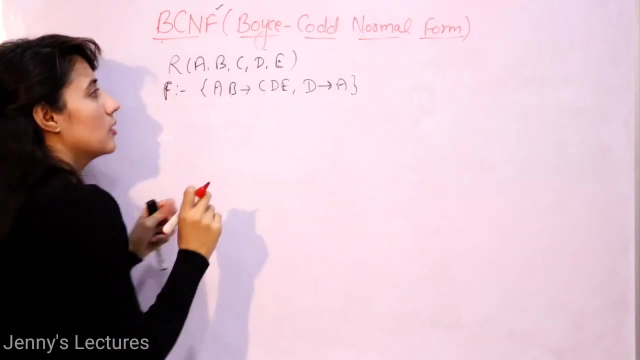 complete, you know link of that complete playlist of DBMS in description box. so you can see that now the highest normal form of this relation is second NF. right, let's take one more example. so let's take this example and check out the highest normal form in this relation. for that you need to find out the candidate. 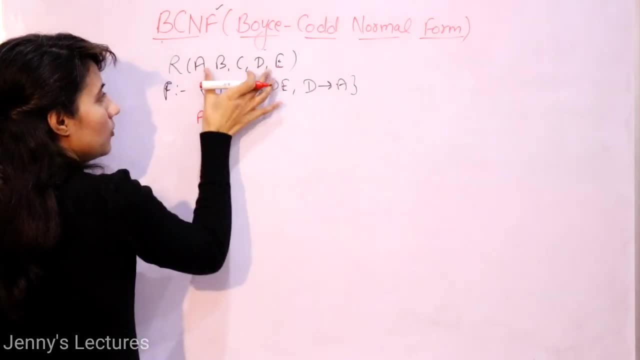 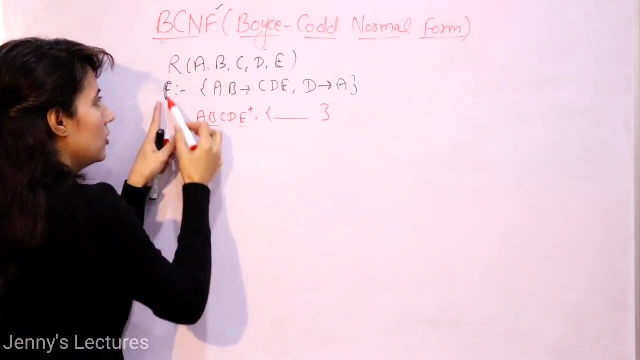 keys. how to find out candidate keys. take all the attribute of the relation. definitely the closer would contain all the attributes. so this is what super key. now try to discard attributes. how to discard, check the functional dependency: AB will determine CD, so I have a, B, so I can discard CD. D determine a, but I you. 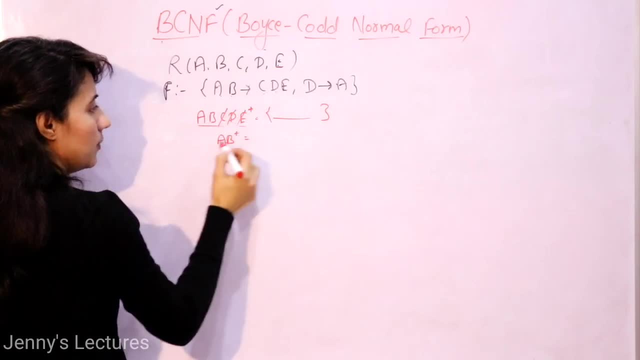 don't have D so I cannot discard anything, so I have now a B. a B is super key. if you still want to find out the candidate keys, then you need to find out the candidate keys and find out. you can find out a B closer. a B closer will have a B reflexivity. 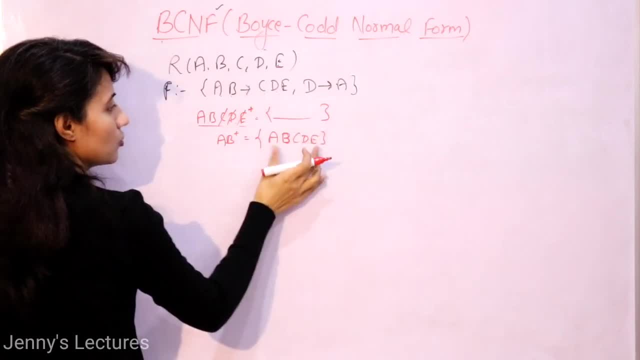 property and if you have a B then you can determine CDE. so it is having all attributes. so a B is what super key now it is, that is that candidate key or not? find out the proper subset. one is a, one is B. closer of a is a, only closer of B. 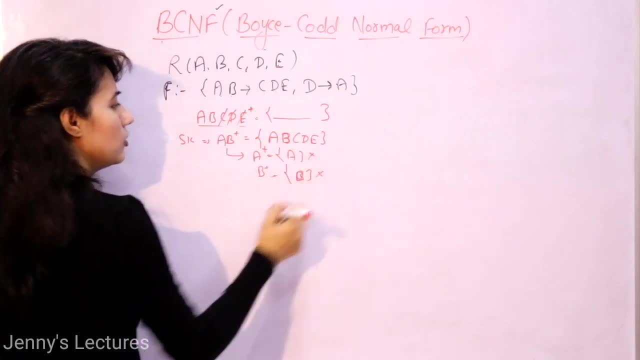 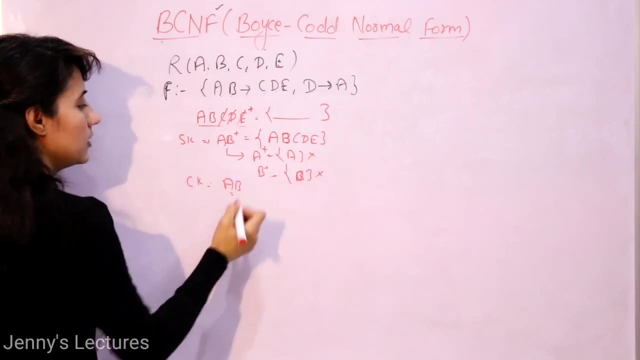 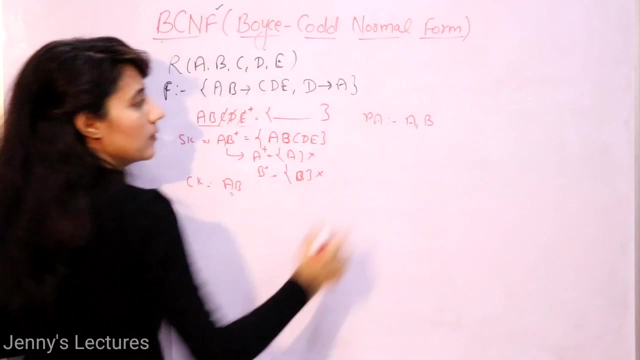 is B only, so it is not super key. it is not super key. so you can say that now a B is candidate key because no proper subset is super key. no, a B is candidate if you go to one candidate key right. so now we got prime attributes, that is a and B. now check out: prime attributes are: 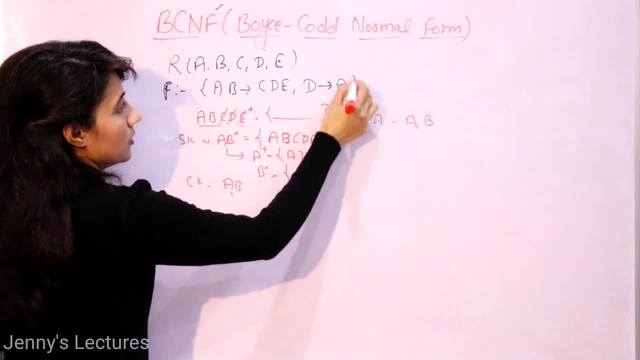 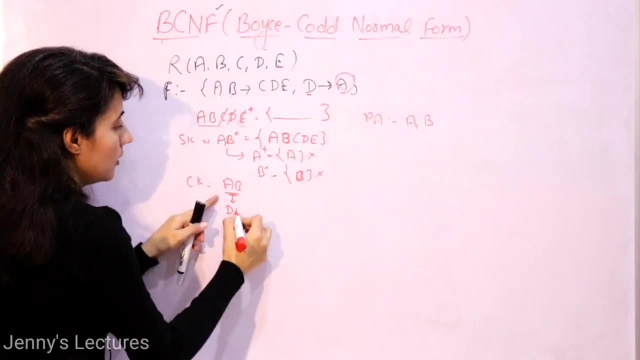 present on the right hand side of any functional dependency or not. yes, here we have a. so now, at the place of a in the existing candidate key, I can replace D. so now I got D B. but I cannot say that it is candidate key. you have to find it. 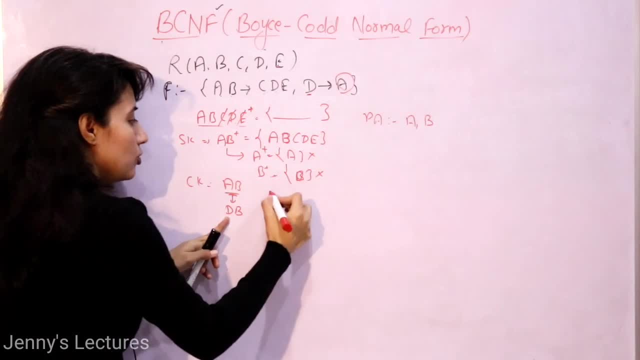 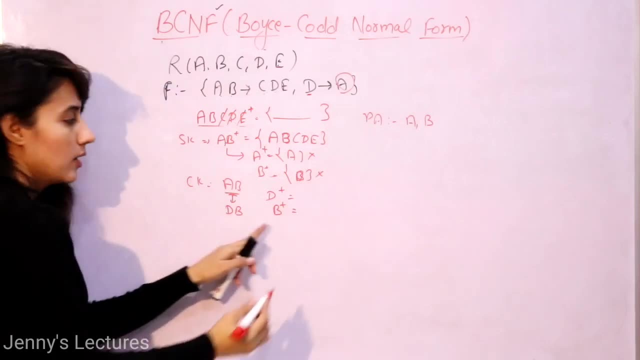 out, but I can say that it is super key. so how to find it out? the closer of it is sorry, this proper subset is D, one is B. find out closer of D, closer of B, but already we have found out B is not super key. now, closer of D, using D, I can find. 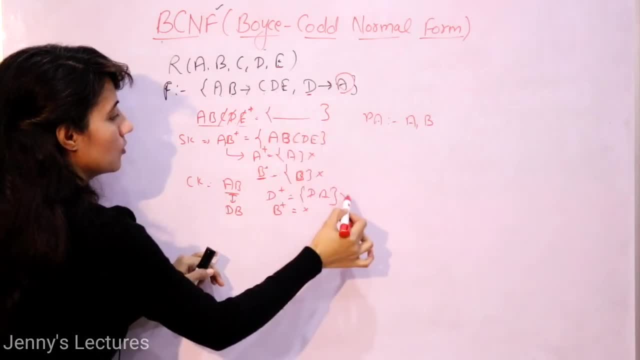 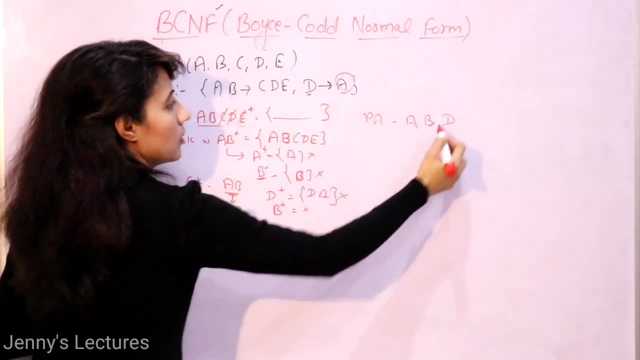 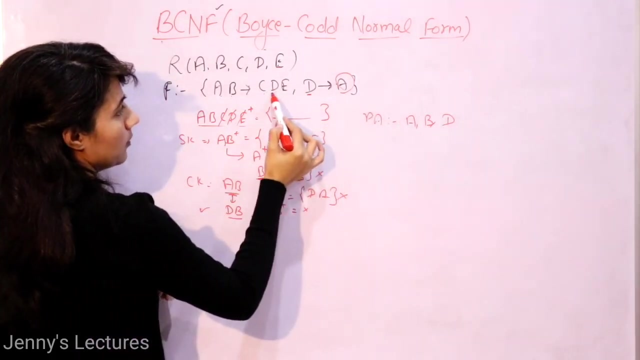 out D and a, nothing else. so it is also not super key. so now you can say that B, D is also a candidate key. so now prime attribute is what? D? one more prime attribute we got, that is D. find out, see, here we have prime attribute D, D is. 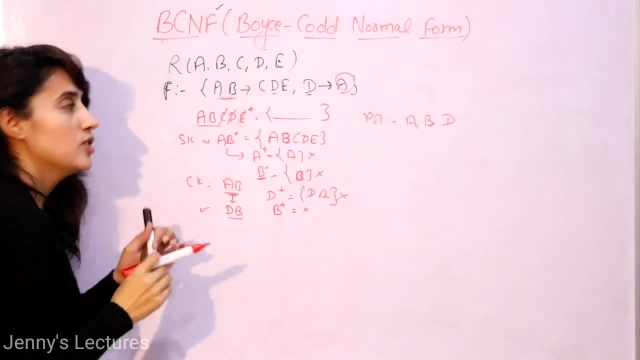 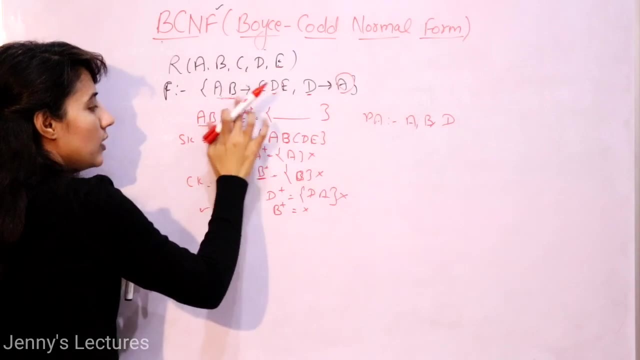 present. on the right hand side of this dependency, right by splitting, I can say that a B determine D, only D, only C, only E. so at the place of D I can replace it with a B. so if you replace it with a B then we have already discussed that a B. 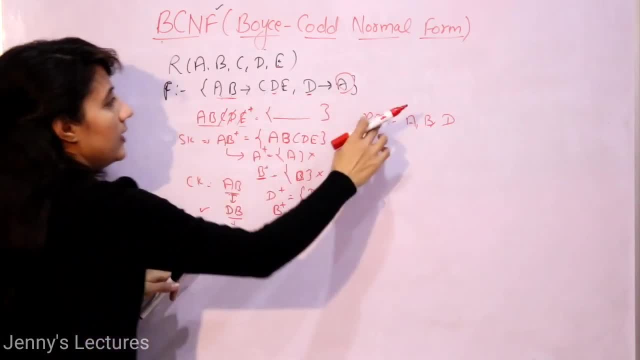 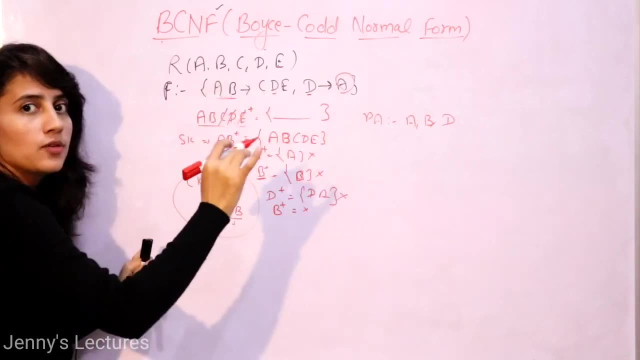 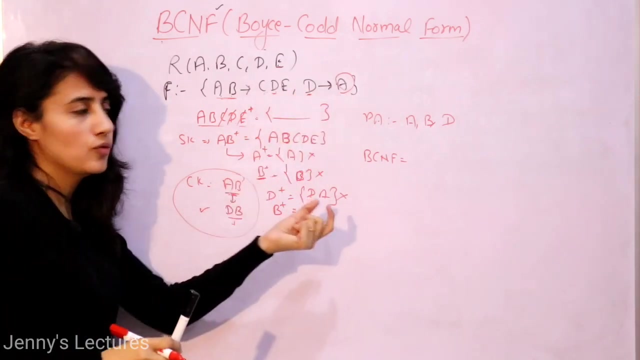 is a candidate key, no need to replace right. so now no more candidate keys. are there two candidate keys? are there a, B and B D? now find out. first of all, we will check for highest. that is BCNF. is it in BCNF or not? for each functional dependency, check out the rules for BCNF, definitely. 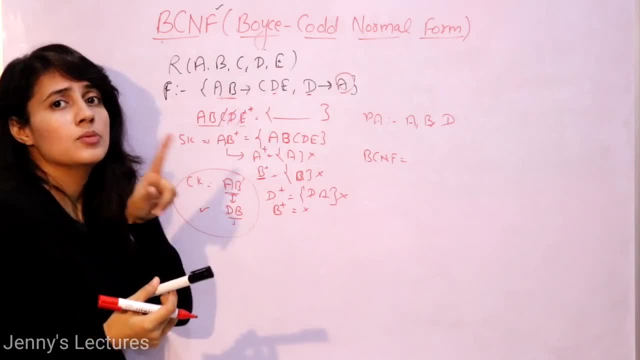 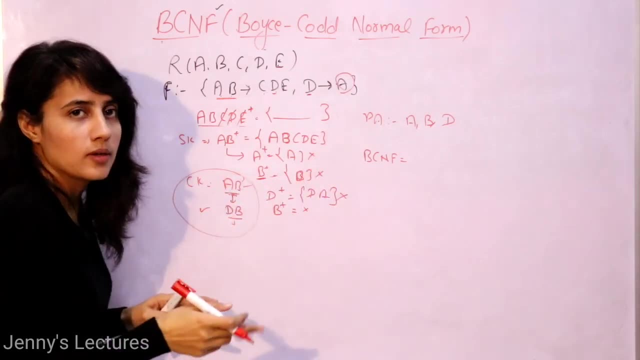 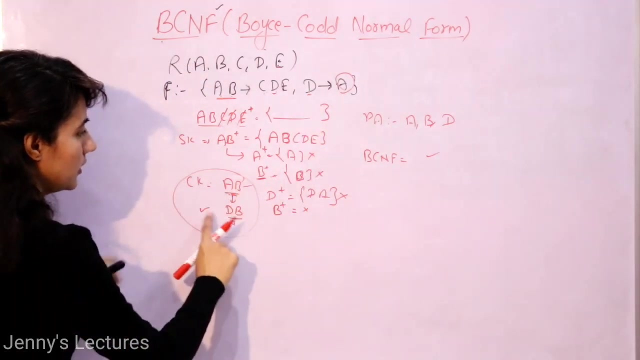 obviously we'll check the that condition that the left hand side must be super key. left hand side of this dependency is a B. is a B super key. a B is candidate key. definitely it is super key. so yes, it is satisfying the property is D super key. is D see D is. 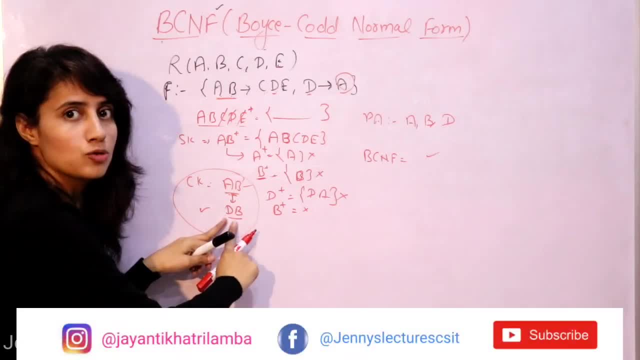 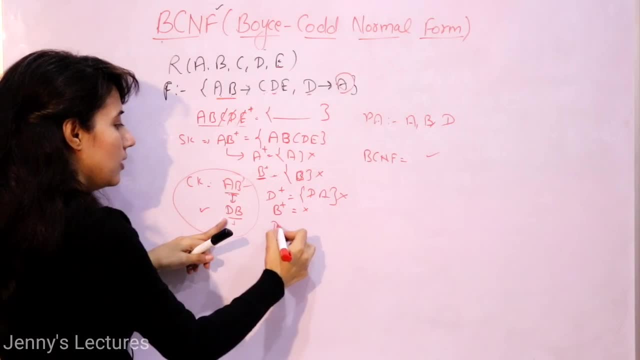 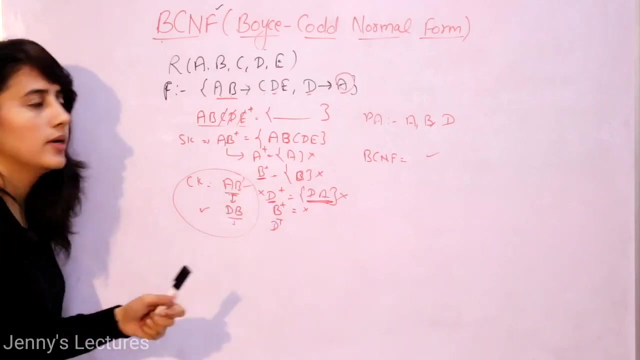 super key. B is candidate key, right? so how alone D can be super key? and if you still want to find out, then you can find out the attribute closure of D. attribute closure of D have we already discussed. it is only DA not containing all the attributes, or D cannot be super key. we have already discussed, right. so now this: 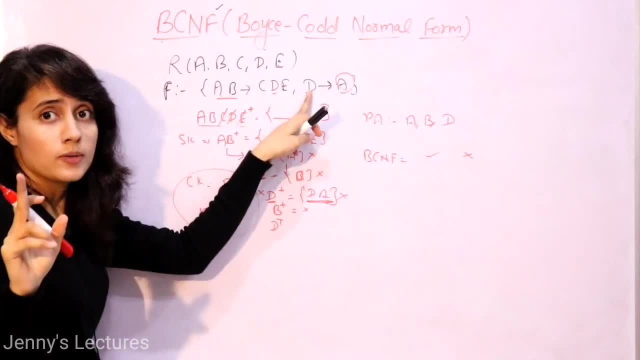 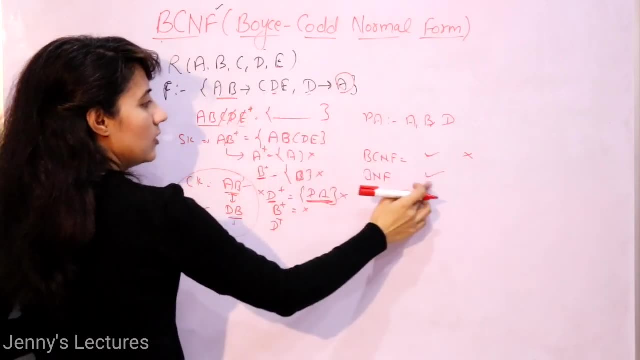 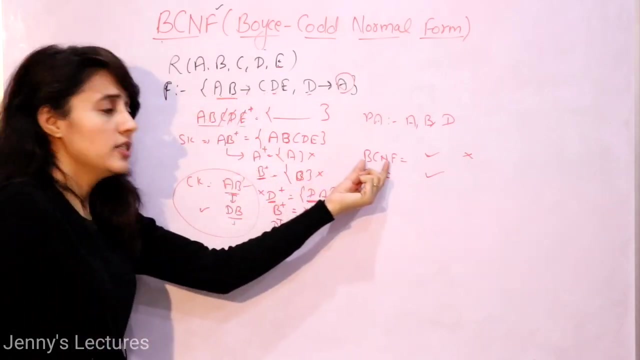 is violating the property of BCNF because left hand side is not super key. now check for third NF. if this is in BCNF, definitely, definitely, this functional dependency will satisfy the rule of DCNF third NF, right, it is not. it is not a transitive dependency, right, because obviously for BCNF. 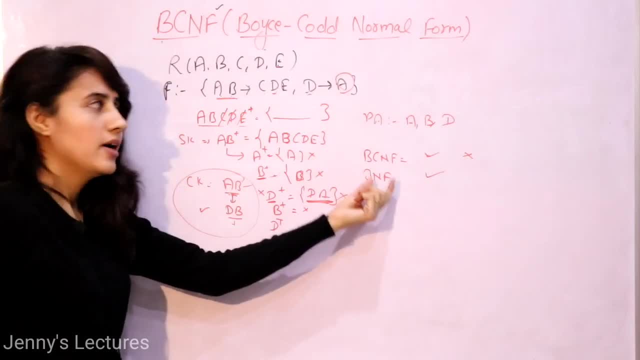 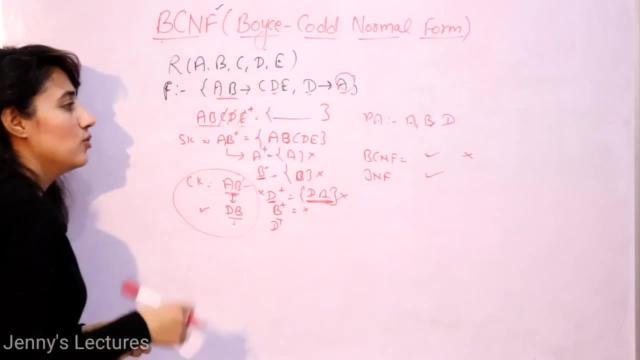 that relation should be in 3NF and if this functional dependency is satisfying the property of BCNF, then by default you can say that it is in 3NF. right? if you still want to check, you can check out. I will check out for this one. only D determines A. is it transitive dependency? because 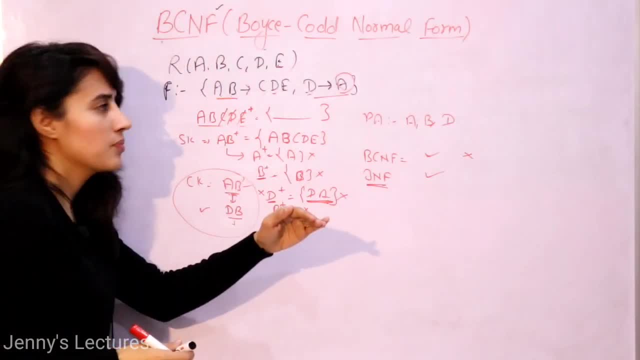 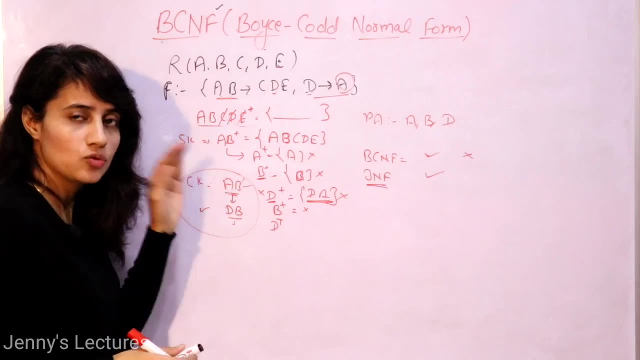 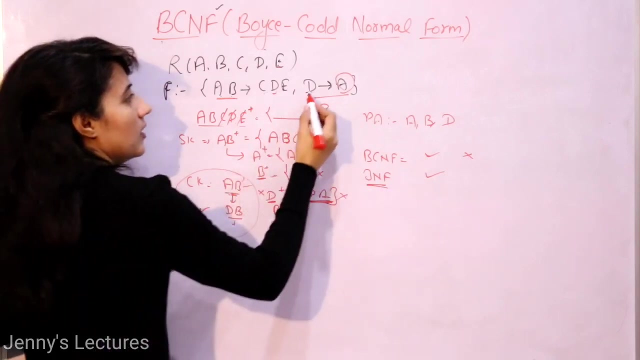 3NF. in 3NF we deal with transitive dependency. so what is transitive dependency? this one, how you will check either left hand side is super key or right hand side is prime attribute. then you can say that that is in third NF. that is satisfying the rules of third NF, left hand side. 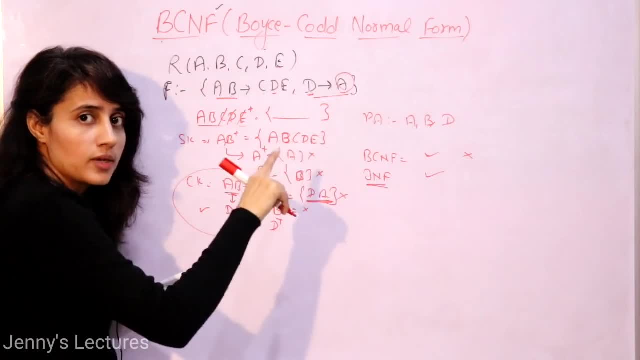 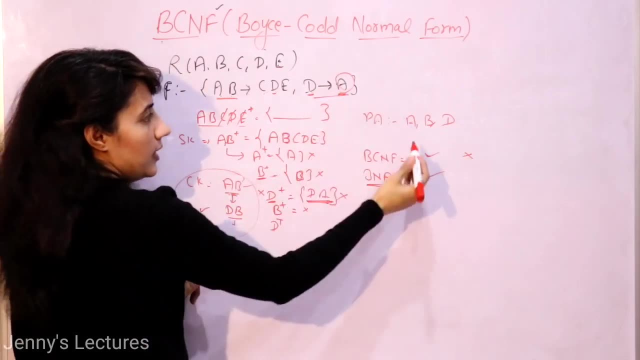 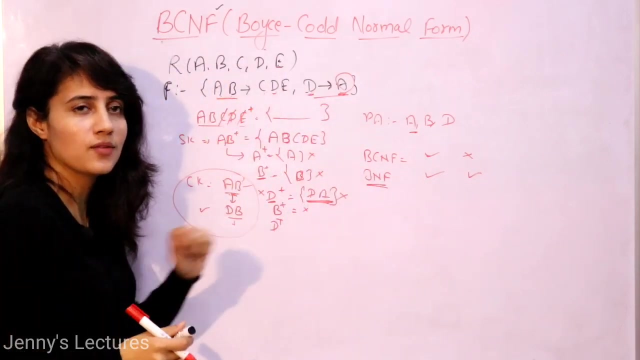 is super key. no, so we have checked for one condition, but check out for second. is this one right hand side, prime attribute? yes, A is prime attribute, right. so this is satisfying the property of 3NF, the rules of 3NF. this is not a transitive. 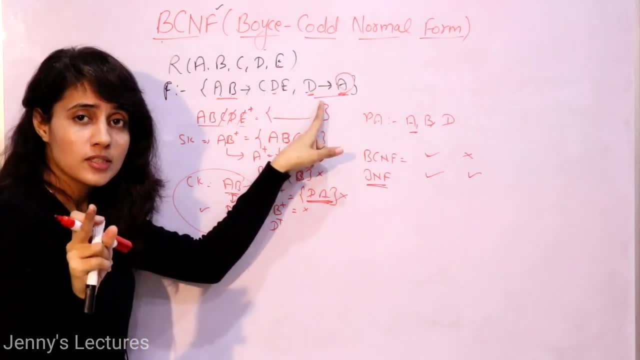 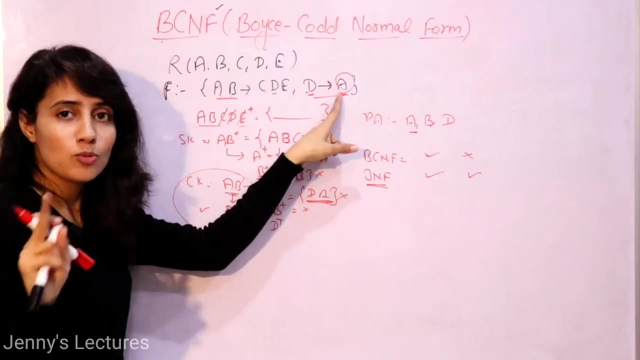 dependency in another term you can say what is transitive dependency, non prime attribute, determining non prime attribute. but this is what? a prime attribute, not a non prime attribute? right, so it is in 3NF, but it is not in BCNF, so definitely would be in second NF and highest. 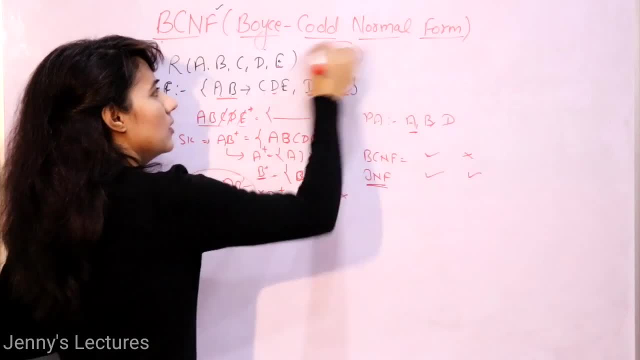 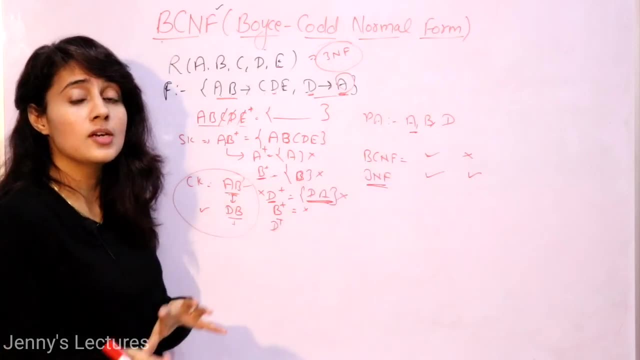 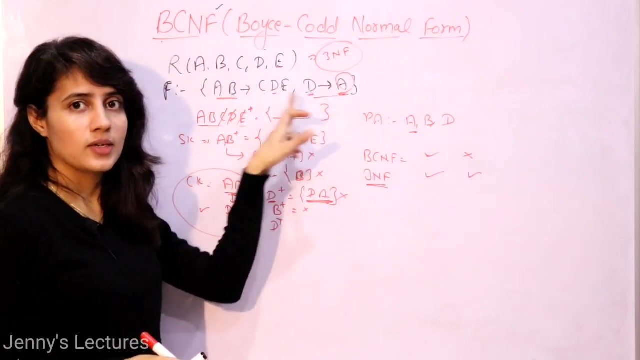 normal form of this relation is 3NF, and and you will find a rare case in which a relation is in 3NF but not in BCNF, because almost every relation which is in 3NF will be in BCNF, right? so this is one of that case when this is in 3NF but not in. 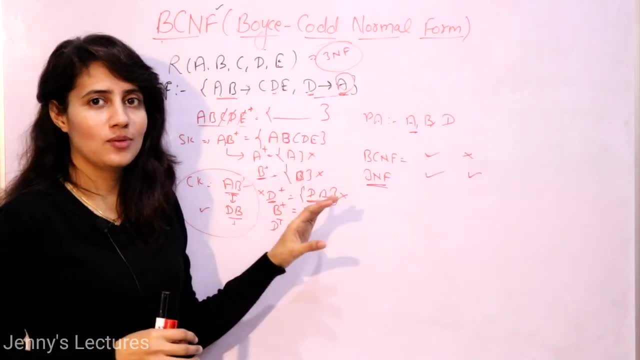 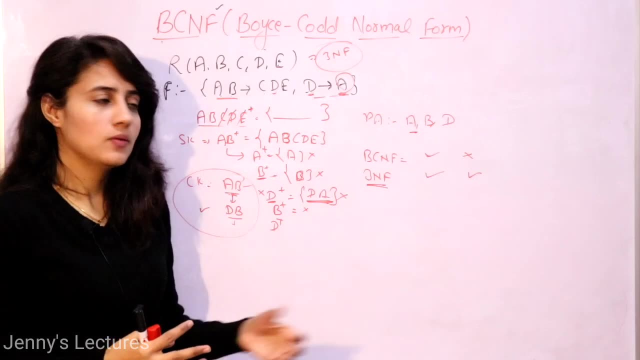 BCNF. so this is all about BCNF normal form, how to find out that a particular relation is in BCNF or not, right? so we also discuss some practice questions like this also. we will take one relation and we will discuss the highest normal form. we will find out the highest normal form in. 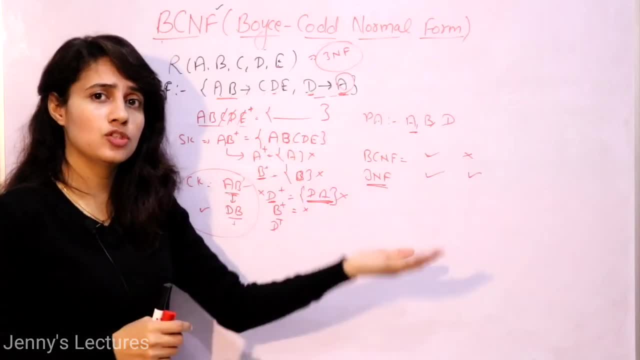 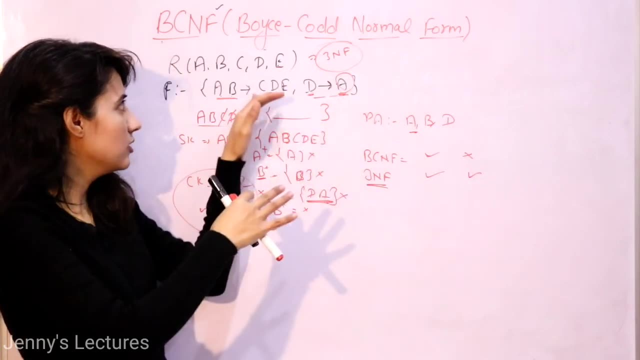 that relation right, some complicated type of questions in the next video, right. and also we will take one table and with help of that table we will not take these type of relation. we will take a proper table with some data and we will find out that particular relation particular. 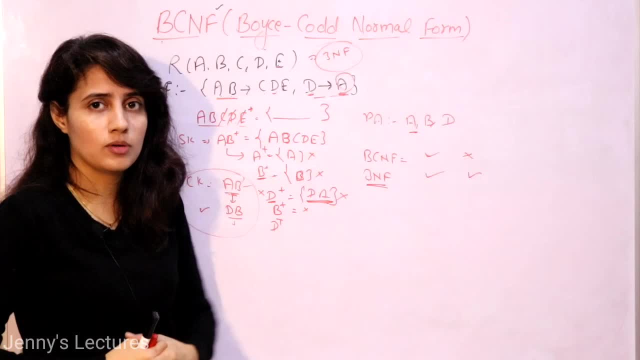 table is in that desirable normal form or not, right so now. I will see you in the next video. till then, bye, bye, take care.